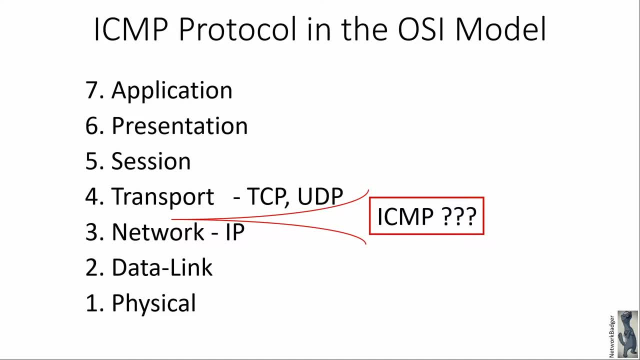 familiar with the 7-layer OSI model. you will not find ping or traceroute in one of the layers, because these tools are hidden under the umbrella of a protocol called ICMP. ICMP stands for Internet Control Message Protocol. Officially, ICMP belongs to OSI Layer 3. right here, However, there is some debate going on about the validity. 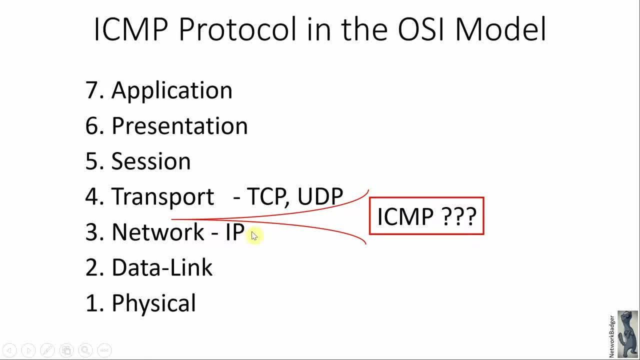 of this classification because OSI Layer 3 is responsible for determining a route or a path through the network in order to get something from source to destination, And the layout of the path is the same if you need to leave the IP address to the дисpenser. 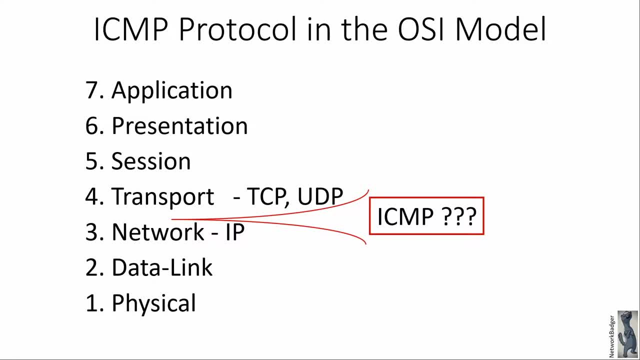 And the layout of the path is the same for OSI Layer 3.. But you should make sure to check the manual before you want to be able to access this database. If you use a complicated the way to access the IP address, you'll have to be careful. 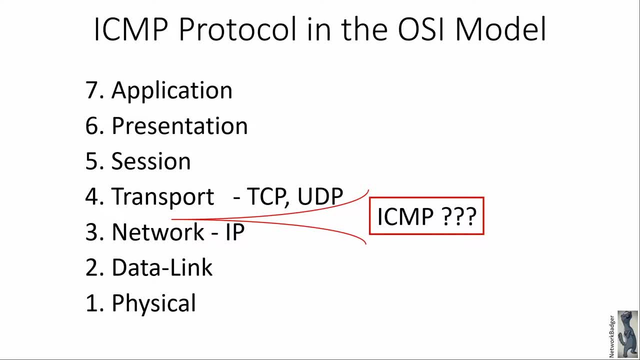 to use an ICMP. So you can see that OSI Layer 3 is also responsible for associated addressing, Usually IP addressing. But ICMP performs none of those functions. It does not determine any route, It has no addressing mechanism and it actually relies on a layer 3 protocol to work. It will not. 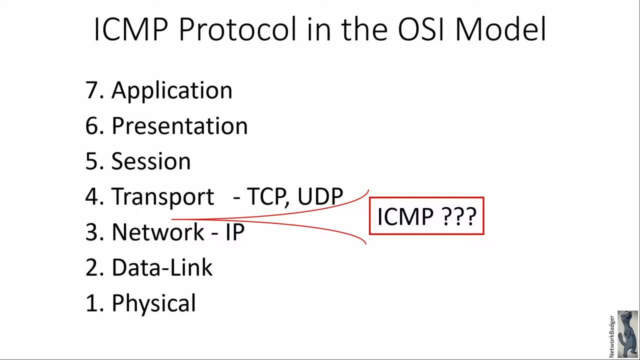 work without the IP protocol. So well, you'll say maybe it belongs to an IP and then it belongs to a particular IP component, And I guess it could work. but for now I can't say for sure, I can't say for certain. 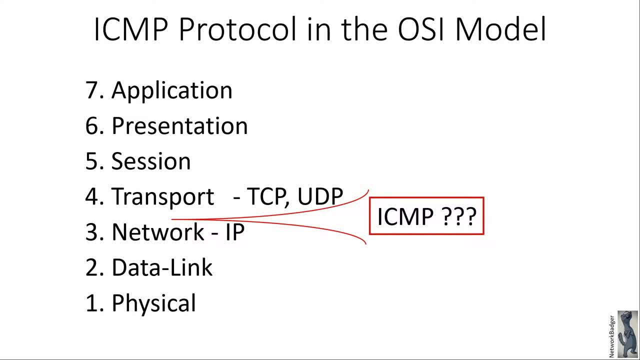 maybe ICMP belongs to layer 4, then Layer 4 ensures that data is transported from source to destination. Layer 4 uses the concept of ports, Layer 4 ports like TCP port 80,, port 443,, UDP port 23,, and so on. But again, ICMP has nothing to do with ports or data delivery. so 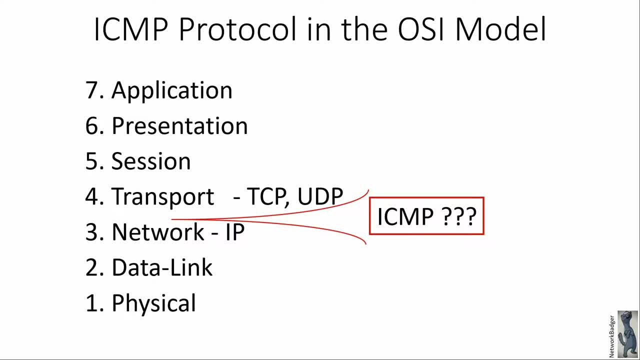 it doesn't belong to a layer 4 either. If they ask you, remember, the official answer is: ICMP resides on OSI layer 3.. If they ask you: is ICMP a layer 4 protocol? Of course not. Is it a TCP or UDP protocol? No, Does ICMP. 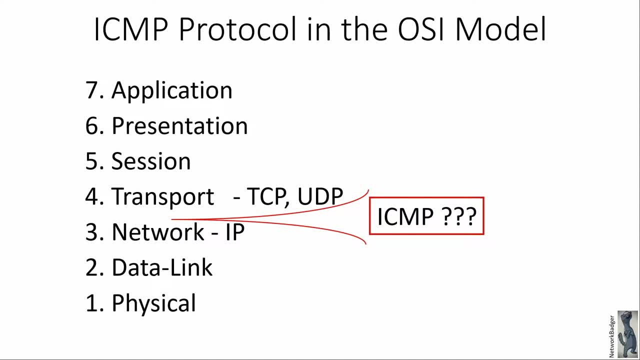 use any layer 4 ports. No, The answer is no, So just keep that in mind. if asked on an exam, if they try to trick you into an incorrect answer, The reason why classifying ICMP is so tricky is that ICMP was not designed to carry user data. 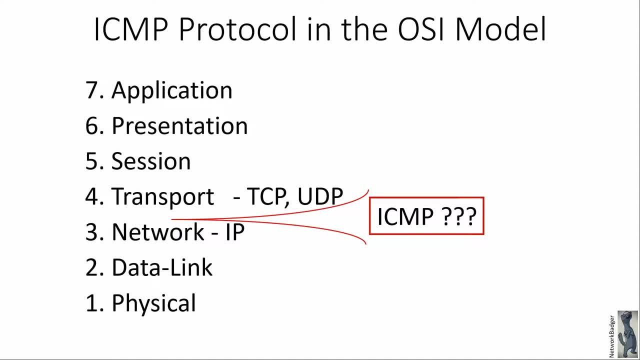 Many protocols are responsible for conveying user data, like web, email, voice video files, etc. But ICMP does not carry any user data. It's an auxiliary protocol. It's a tool used by users and systems for signaling, reporting the state of the network, and so on. When I say users, I mean 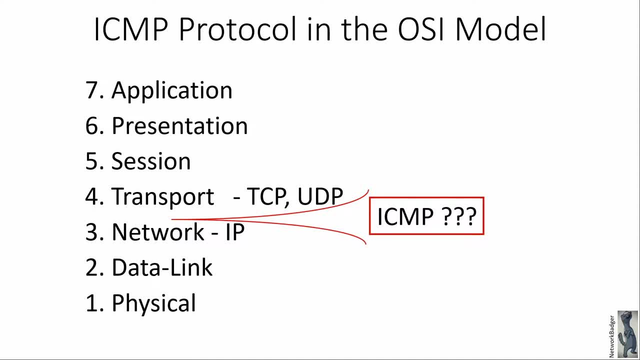 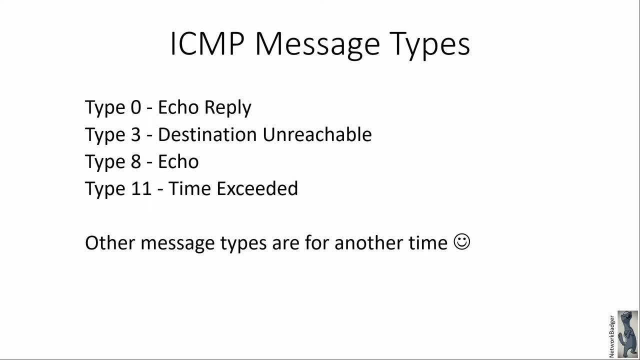 both human users and machines like computers, servers, routers and so on. So when looking at ICMP specifications, you will not find any mention of ping or traceroute. Ping and traceroute are unofficial terms for tools that are built with ICMP messages. ICMP has 256 message types. 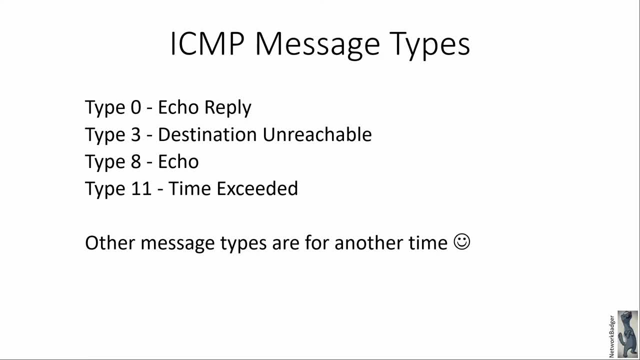 most of which are unused, reserved or depreciated. For now, we're only interested in 4 message types: Echo reply destination unreachable. echo request and time exceeded. They have their own unique message type numbers: Type 0,, 3,, 8, and 11.. With these 4 message types we can build successful. 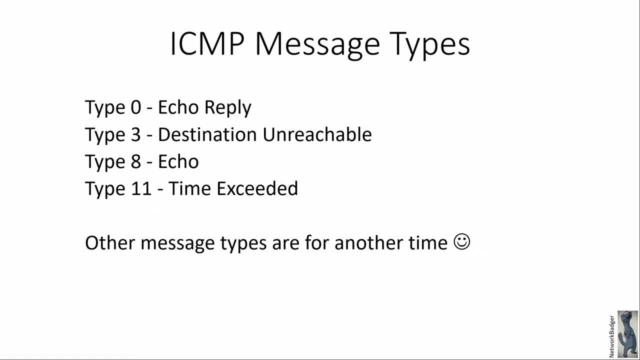 pings and traceroutes. These are like little building blocks for our pings and traceroutes. When you type ping on your computer and press enter, your computer will send out an ICMP echo message, Message type 8.. That's it. That's how your ping goes out. Of course your echo request will be encapsulated in a standard IP. 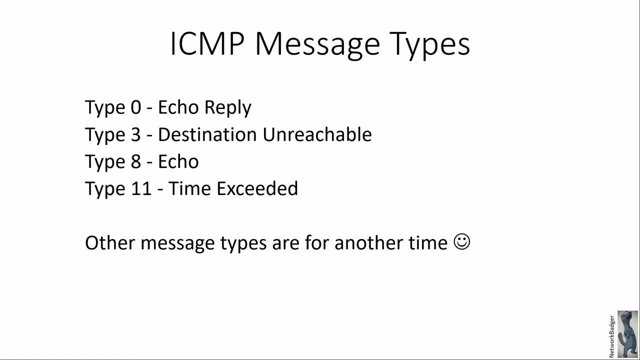 packet containing the source and destination IP addresses, And there will be 3 possible replies that you may receive in response to your echo request message. Or the fourth possible outcome is no reply at all. right, So you may either receive no reply or you will get one of three. 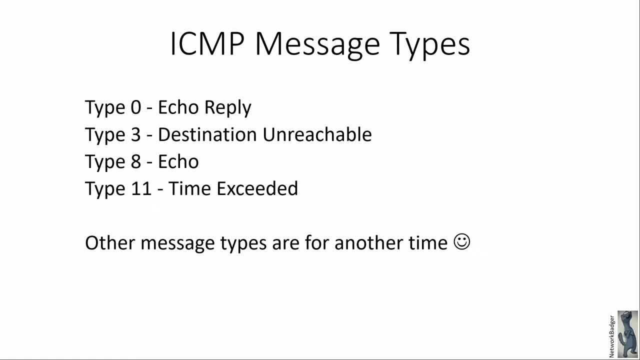 possible reply messages. No reply at all means that your request never reached the destination or the response from your target never made it back to you. No response can also mean that ICMP is disabled on the device that you're trying to ping. That's pretty common for security reasons. 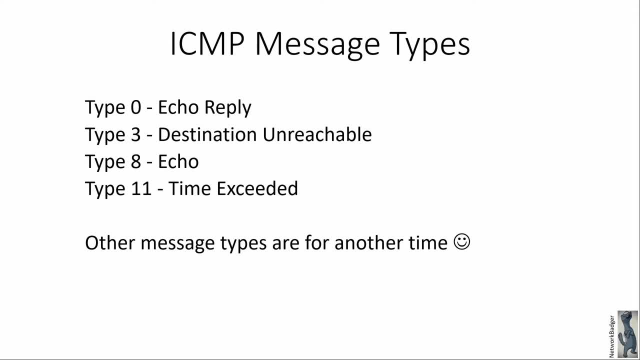 Computers may have some draconian firewall enabled that blocks all ICMP, including pings. I recall Windows firewalls were like that. Now they got a little smarter and they don't block ping by default. but I remember they used to do that If you wanted to ping a computer you had to disable the Windows firewall on that computer. 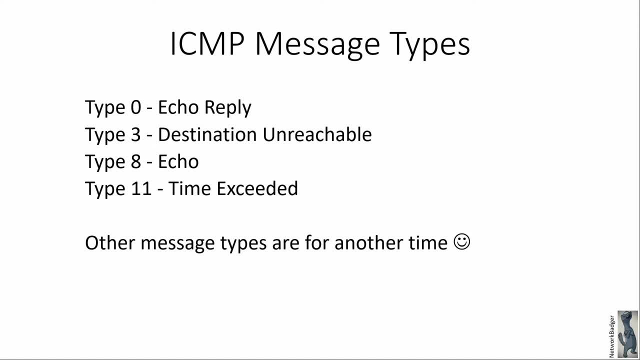 It's a common practice to disable, rate limit or de-prioritize ICMP on critical network devices like switches, routers, firewalls. You may want your device hidden from hackers or bad guys or script kiddies. If you're not familiar with the term script kiddies, these are like amateur hackers, not real hackers. 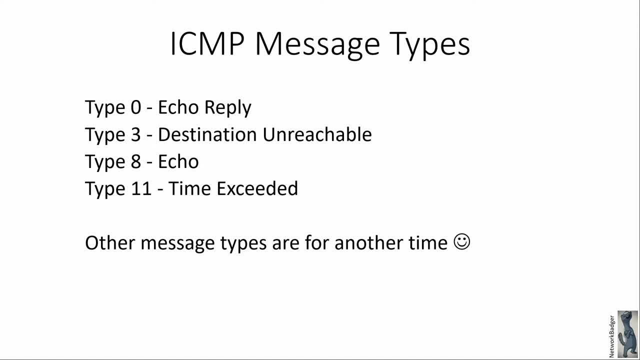 who just got their hands on bad, stupid tools and used them to harm other people without a real purpose or without real knowledge or understanding of what they're doing. So you may want to hide from those guys by blocking ICMP, disabling ICMP on your device. 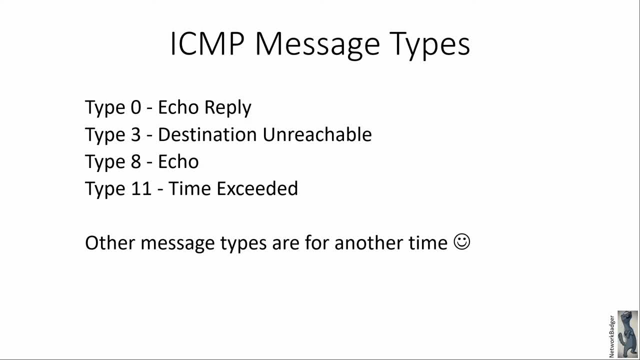 Or sometimes you will notice a device will respond to a few of your pings and then it will stop responding. That way administrators are trying to conserve CPU resources and avoid spending CPU capacity on unnecessary tasks. So remember: unsuccessful or slow pings may simply mean the ping target does not want to bother responding to you. 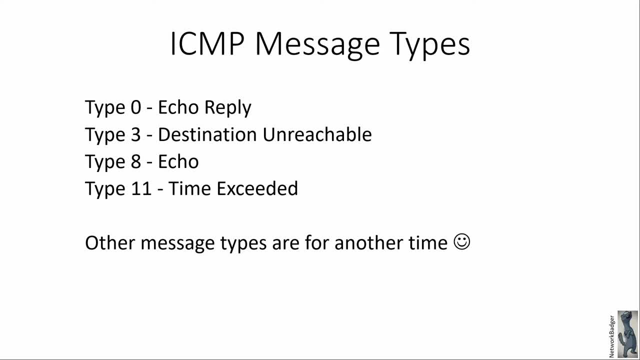 Which doesn't prove there's a network problem. But by default, most routers and computers will respond to pings. But by default, most routers and computers will respond to pings. But by default, most routers and computers will respond to pings. 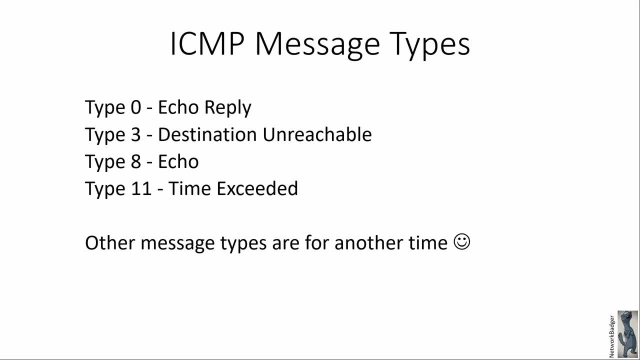 And firewalls by default will not respond to pings. And I don't mean like application firewalls, Windows firewalls, I mean like hardware firewalls, firewalls, firewalls. Those will not respond to pings by default. Of course you can explicitly allow ICMP and then they will respond. 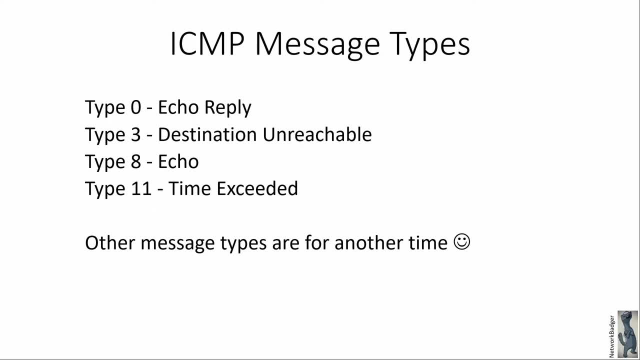 Of course you can explicitly allow ICMP and then they will respond. So So, No reply, No reply. The next possible outcome to your ICMP echo request is actually echo reply. The next possible outcome to your ICMP echo request is actually echo reply. 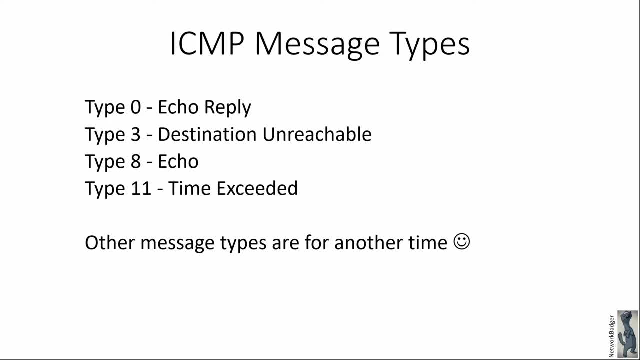 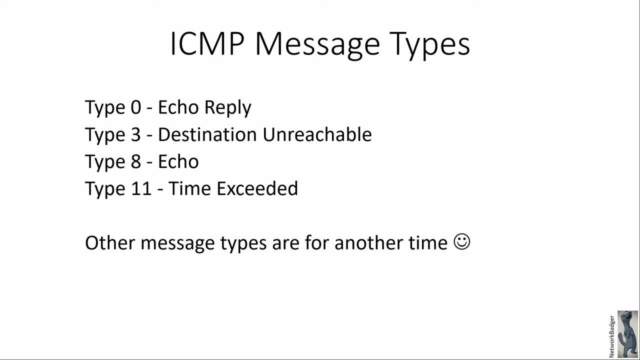 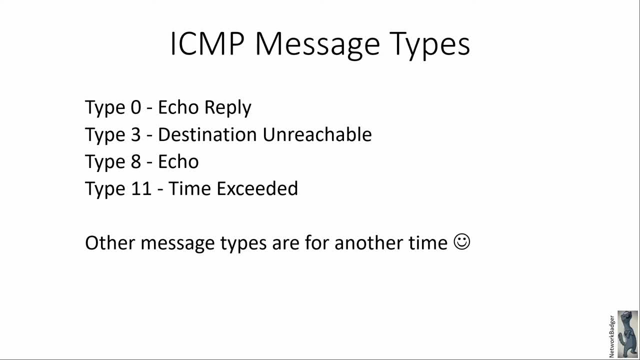 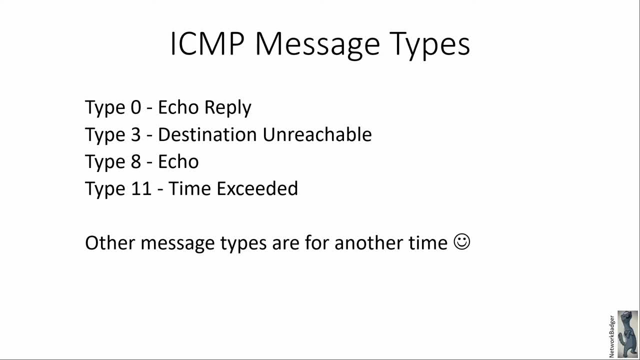 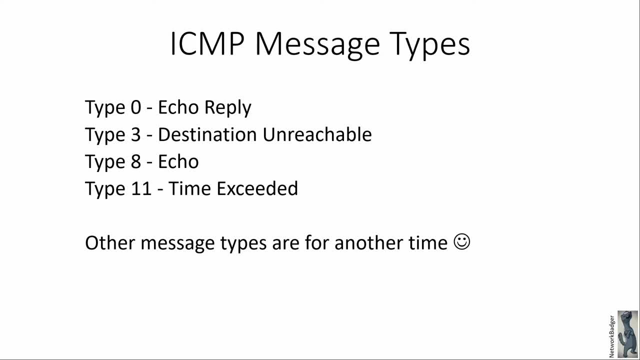 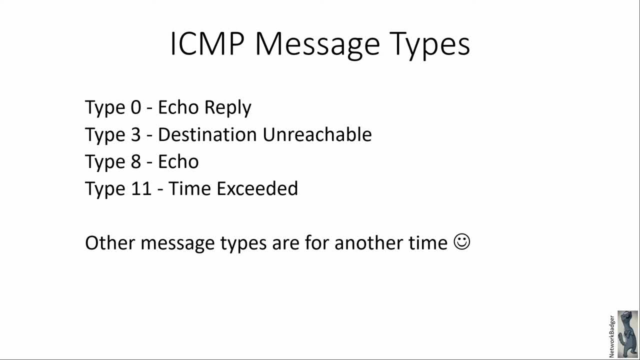 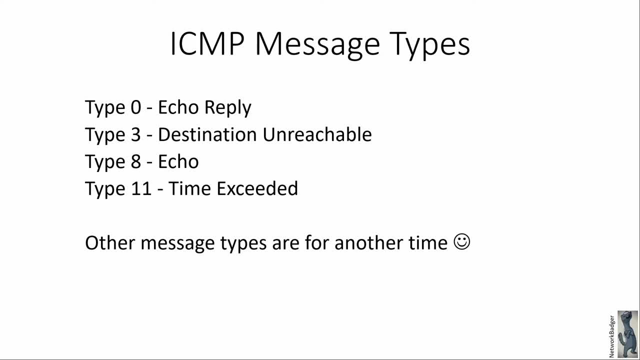 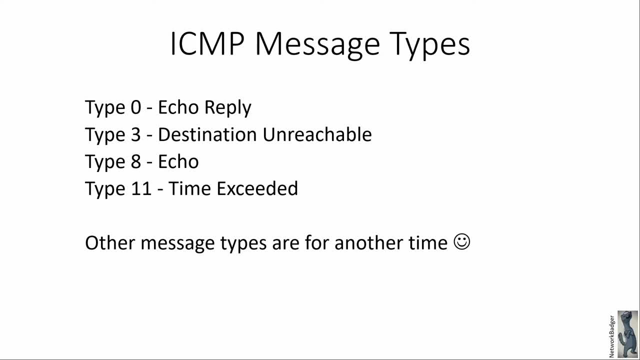 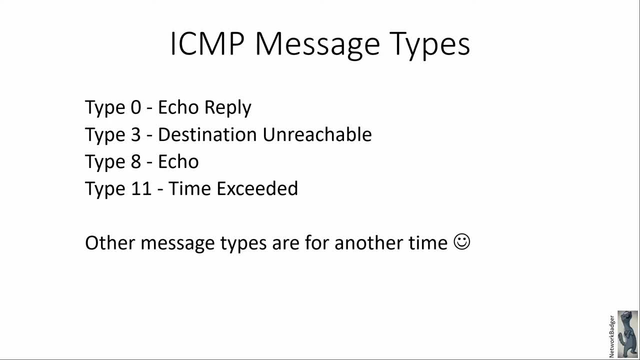 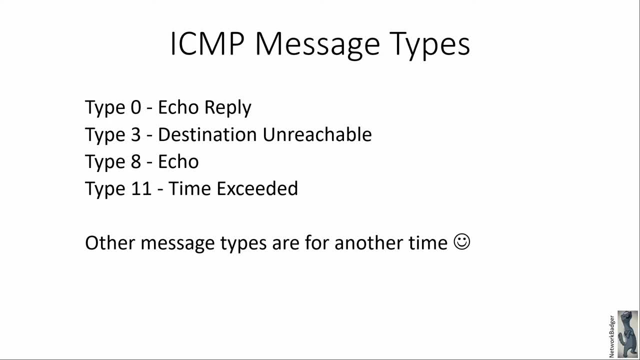 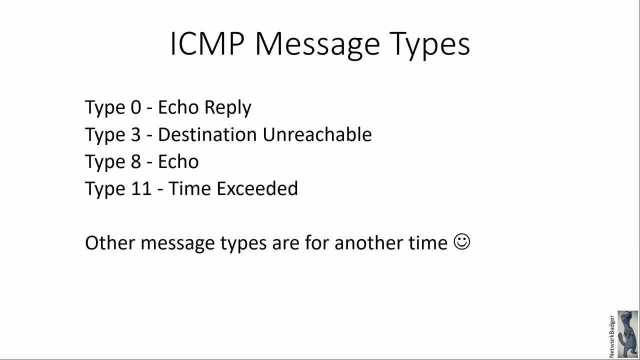 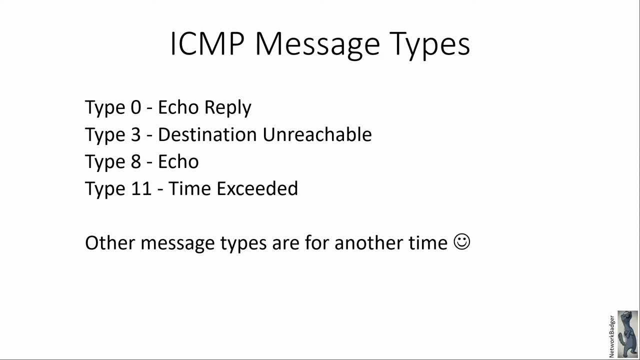 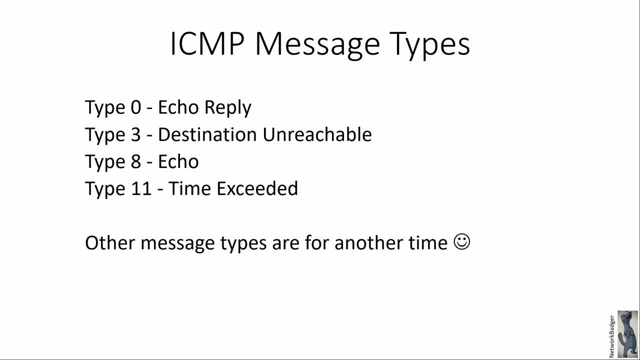 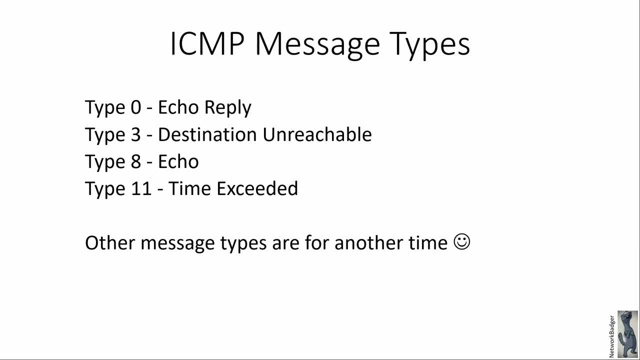 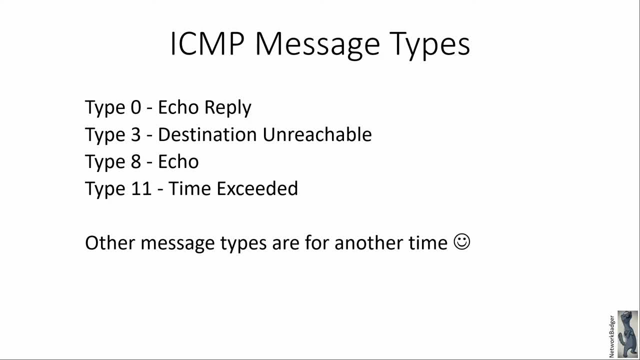 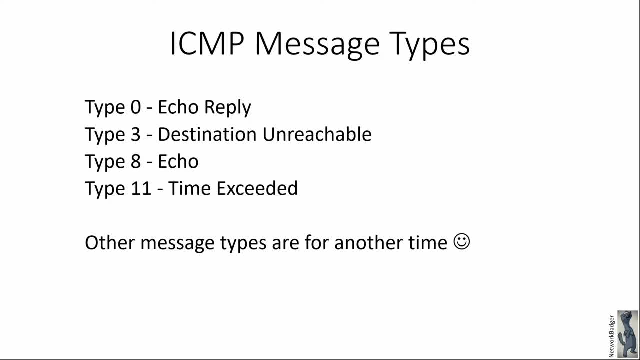 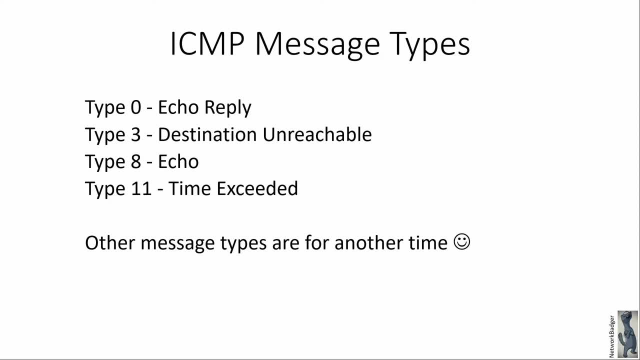 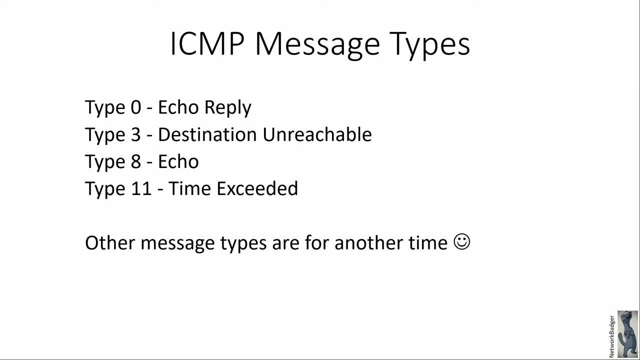 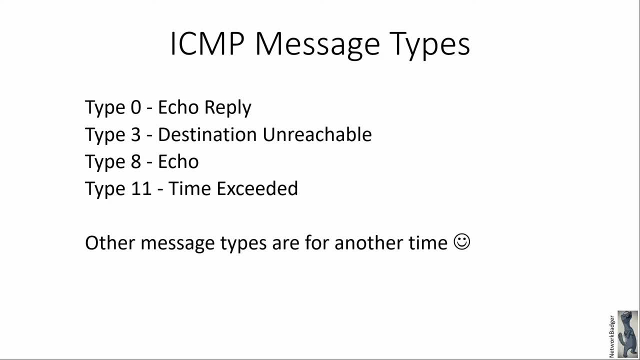 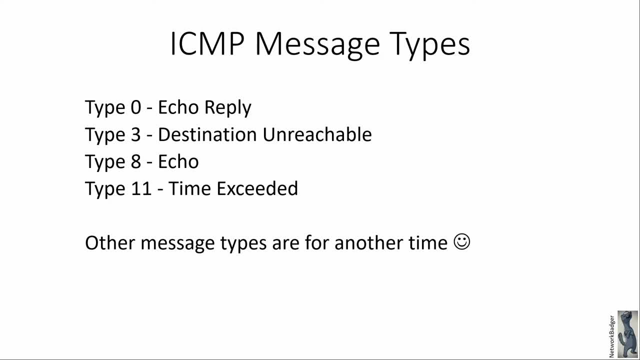 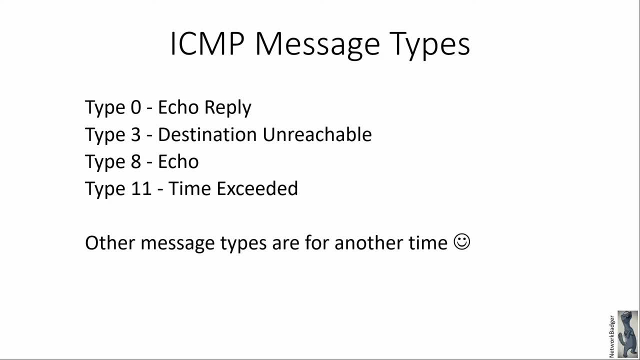 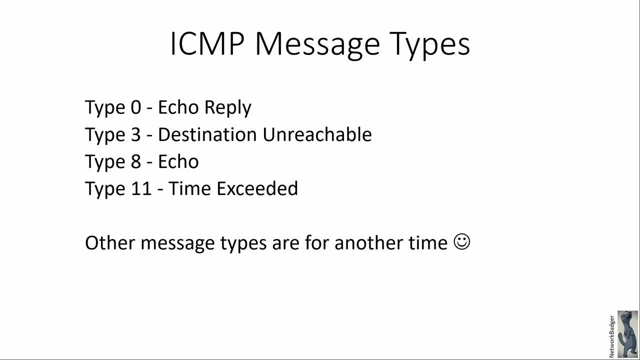 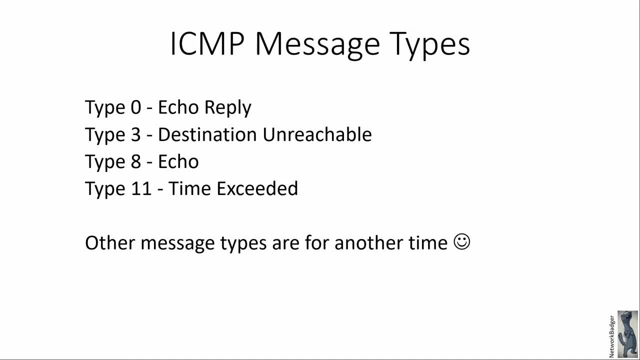 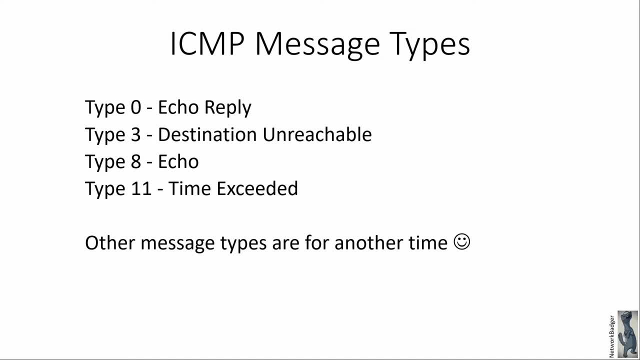 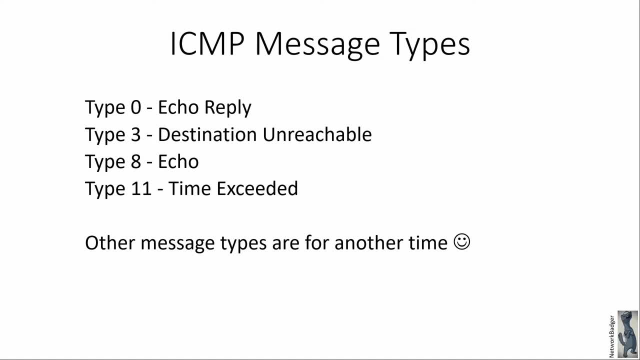 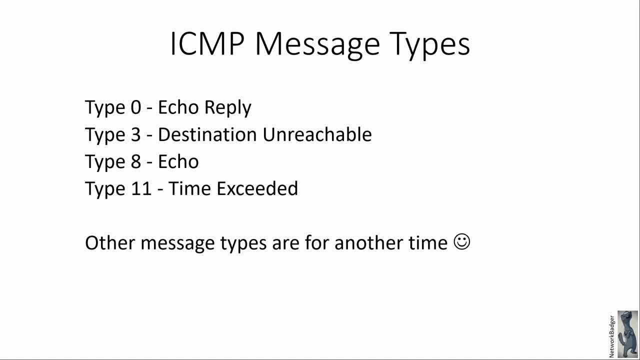 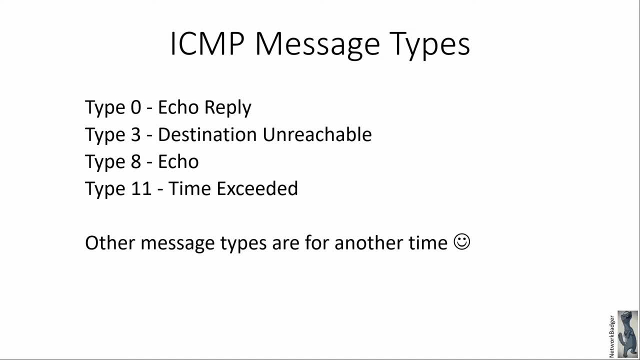 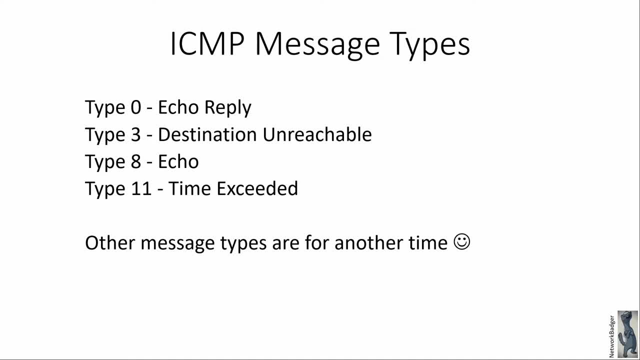 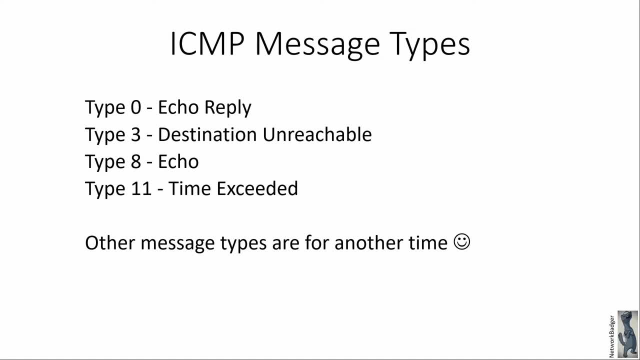 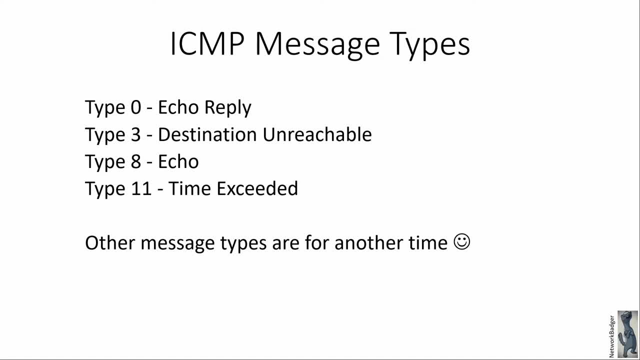 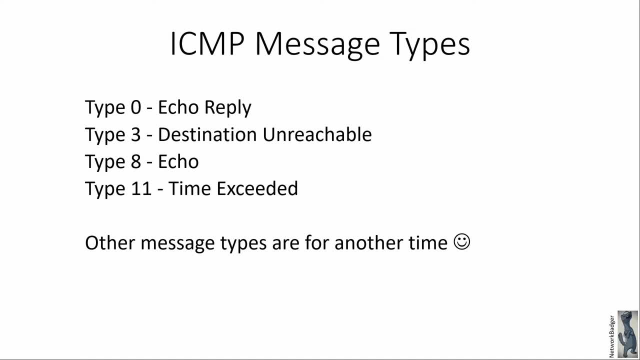 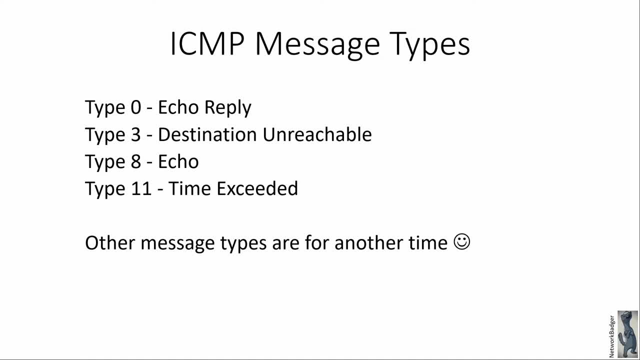 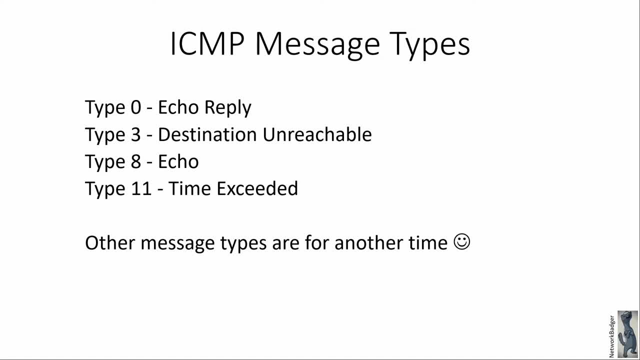 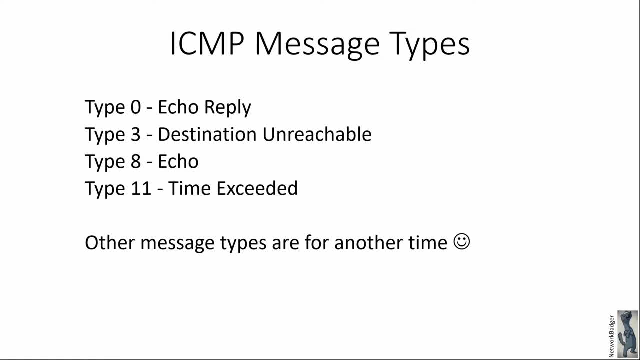 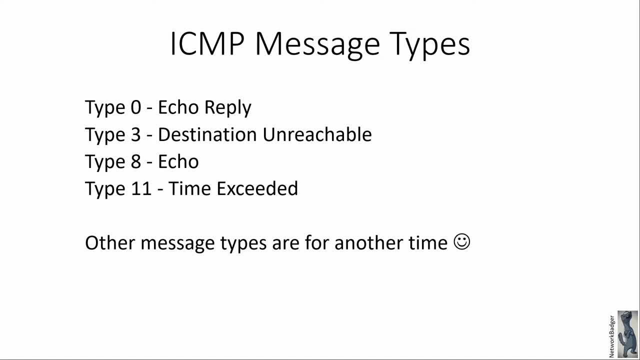 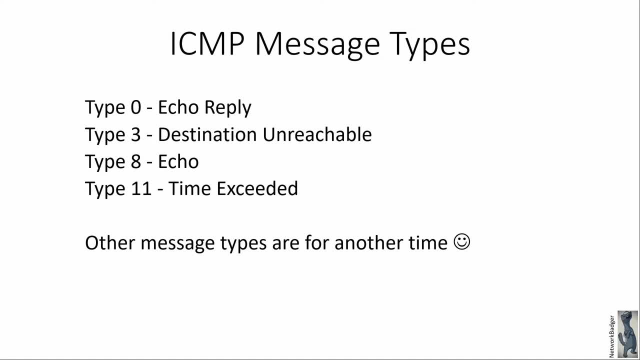 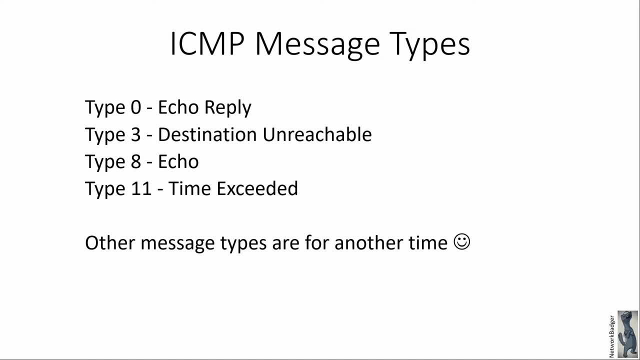 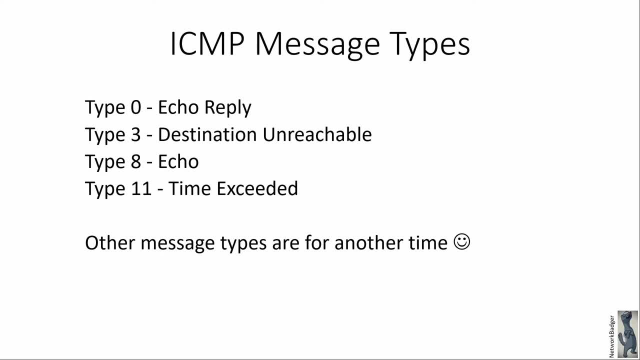 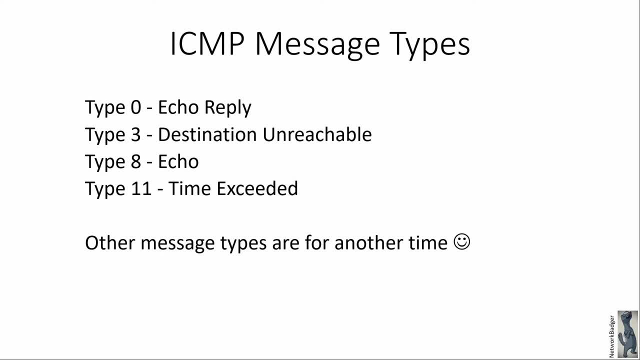 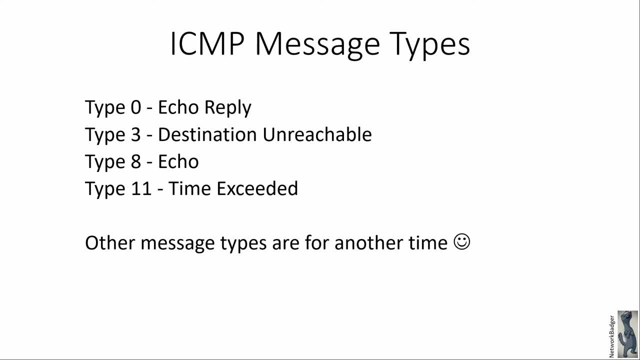 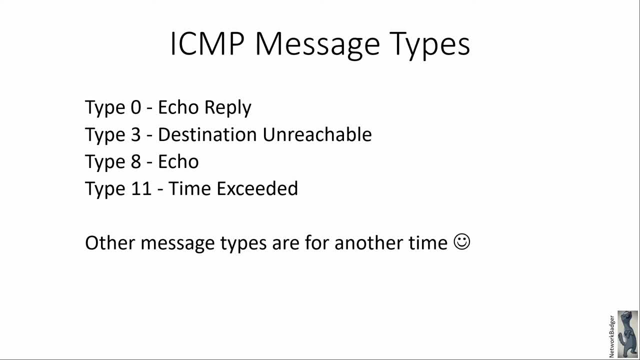 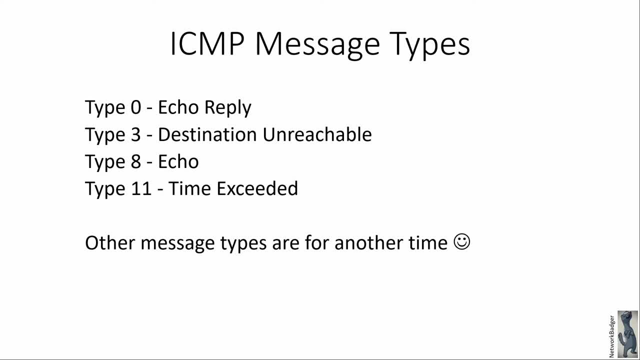 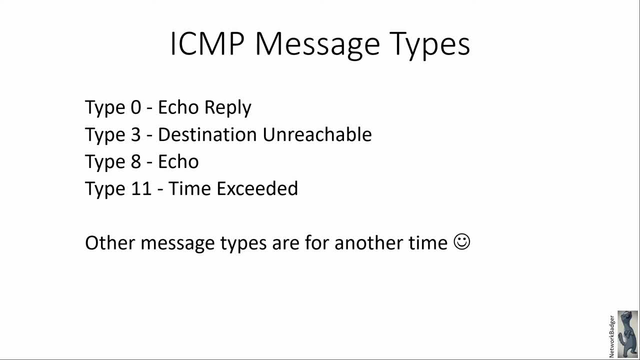 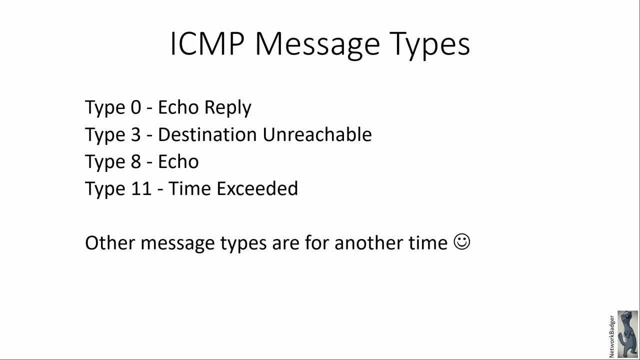 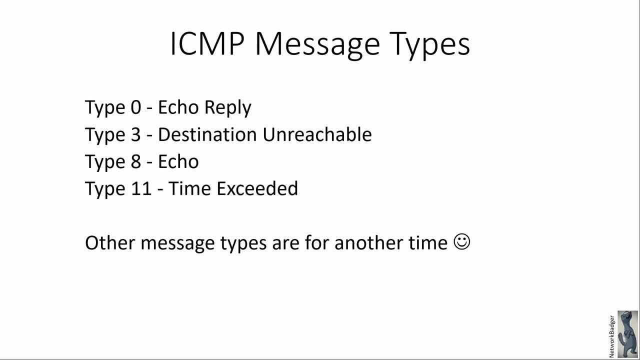 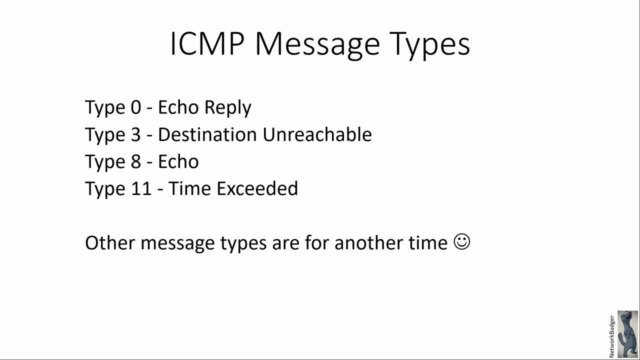 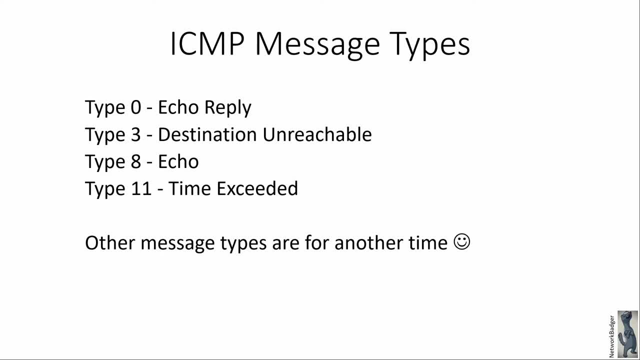 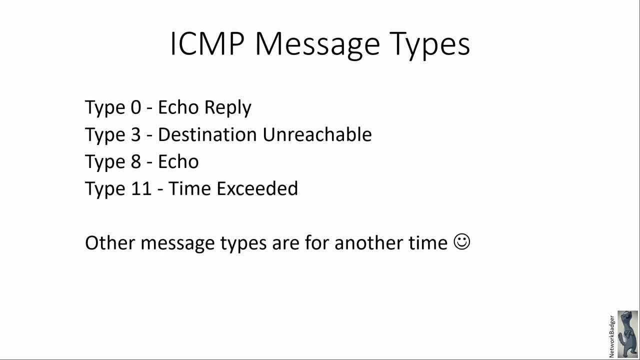 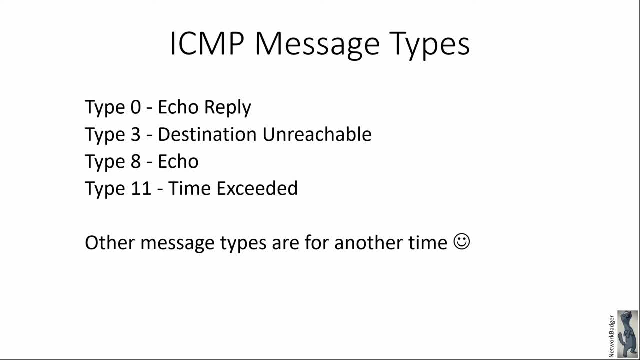 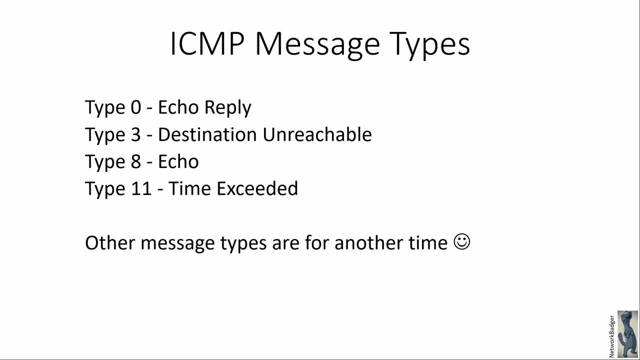 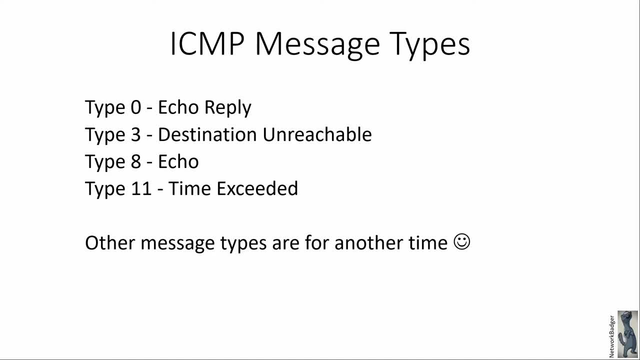 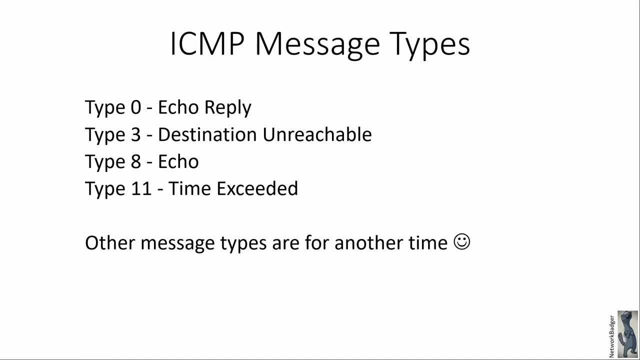 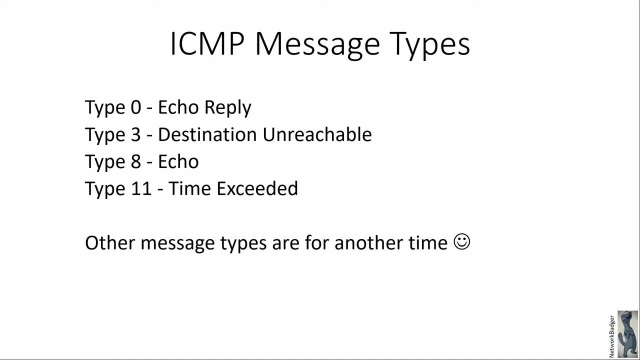 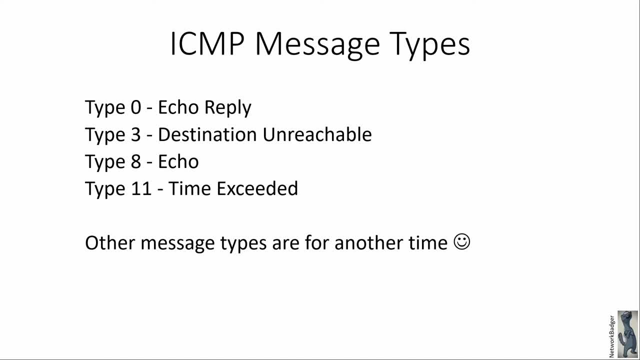 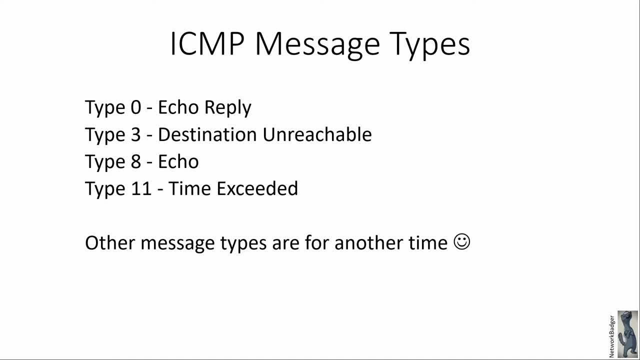 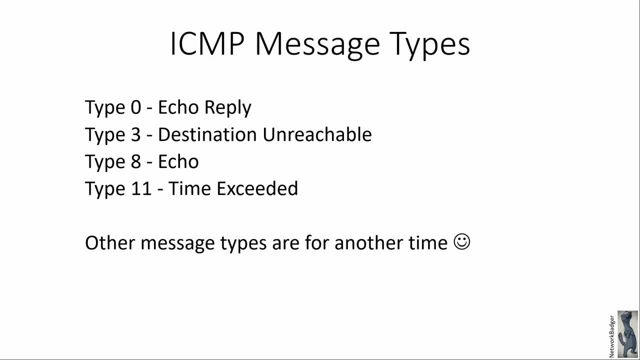 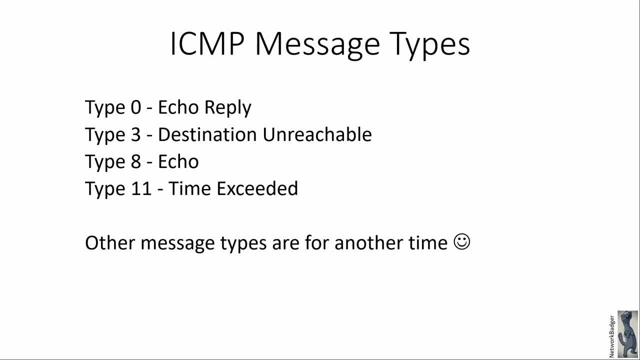 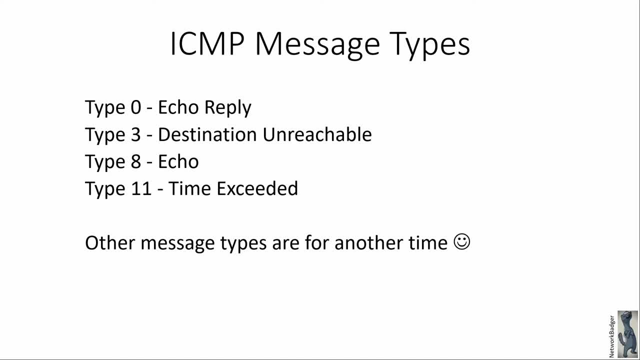 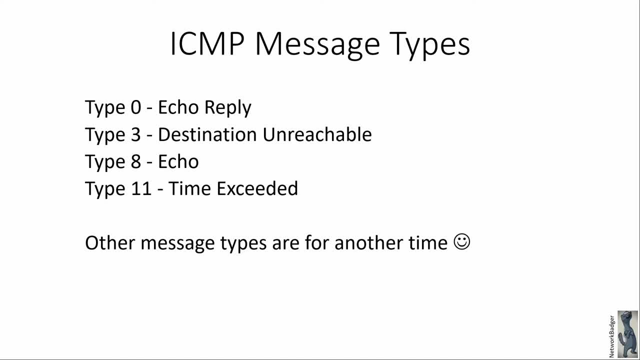 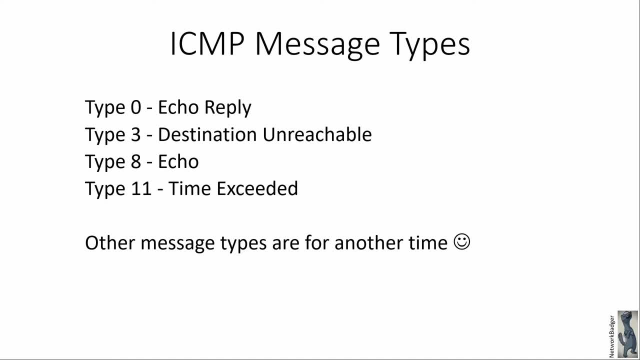 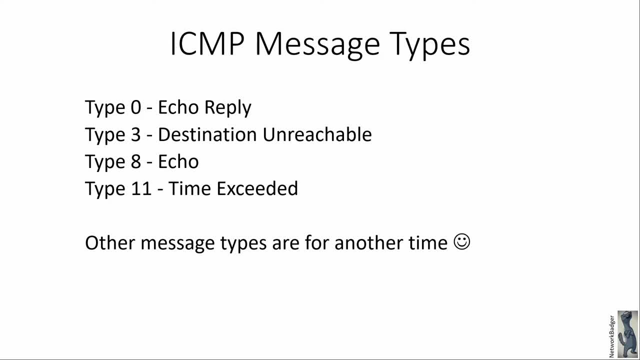 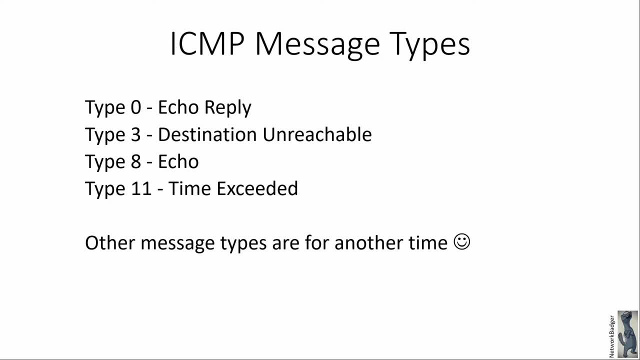 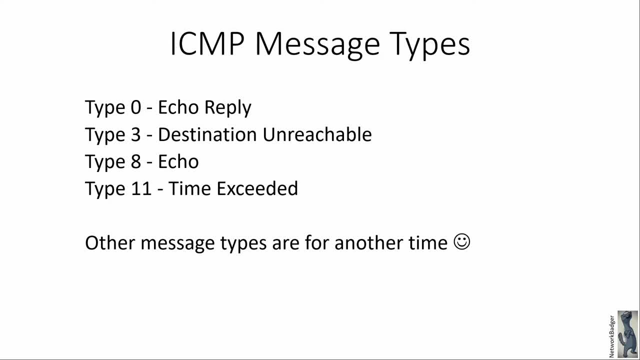 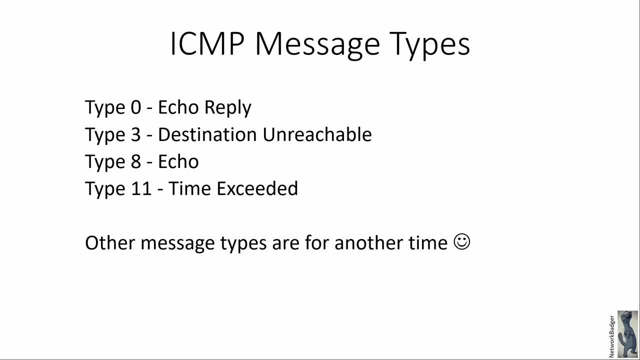 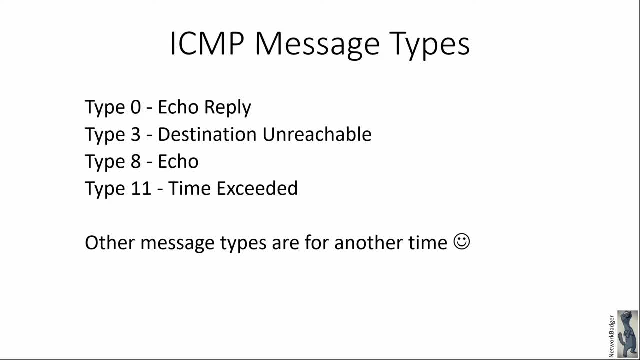 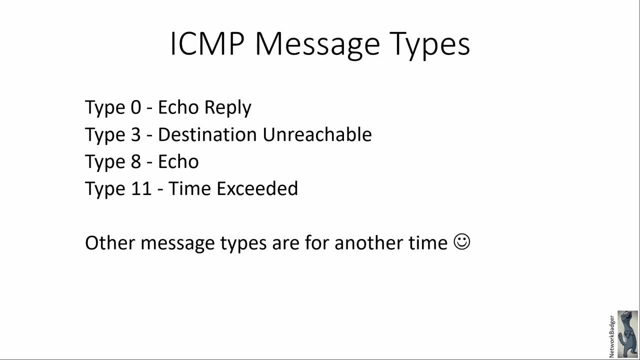 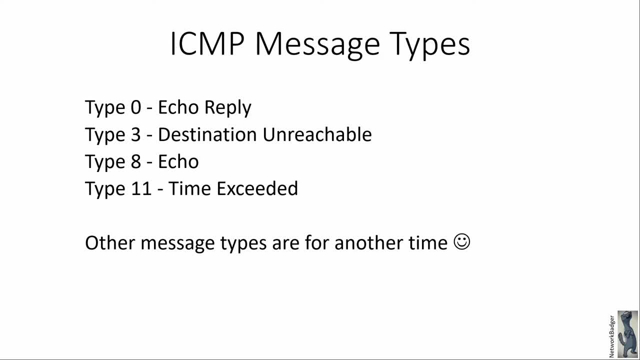 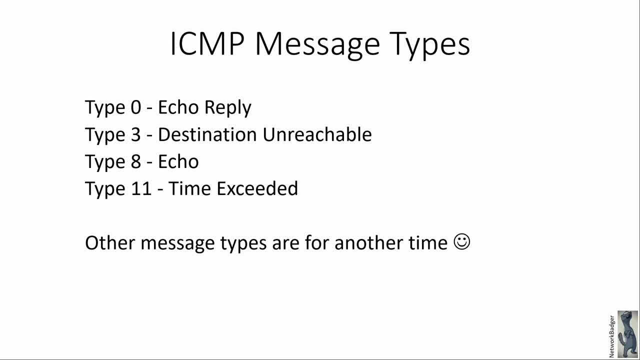 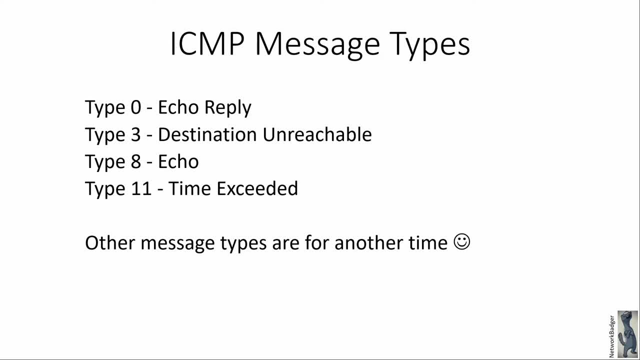 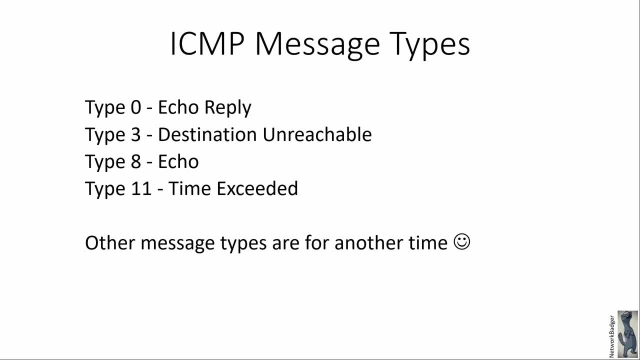 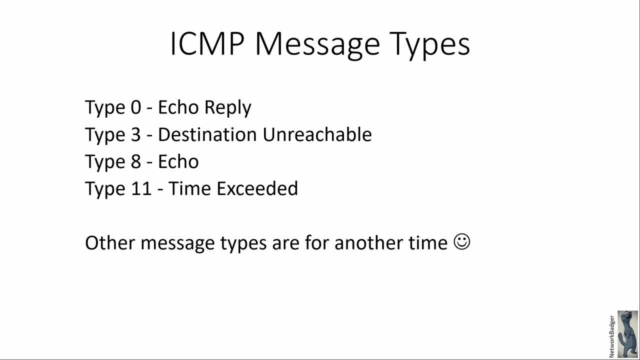 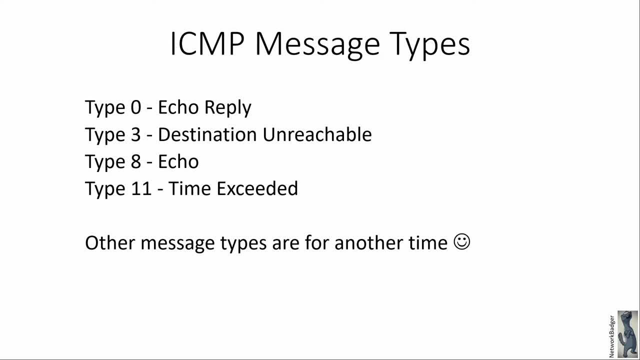 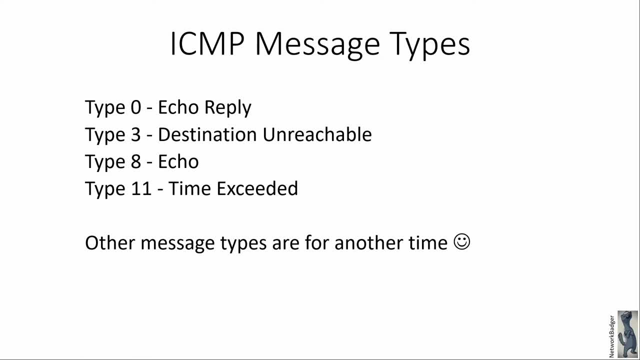 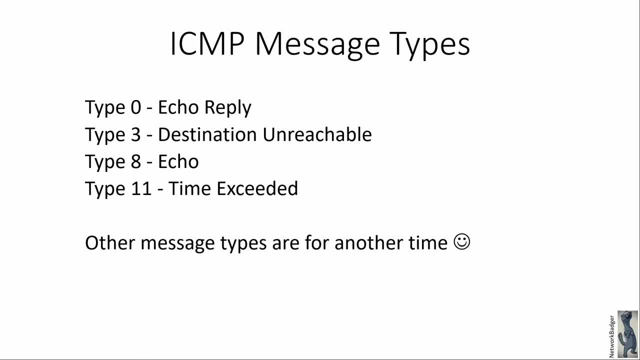 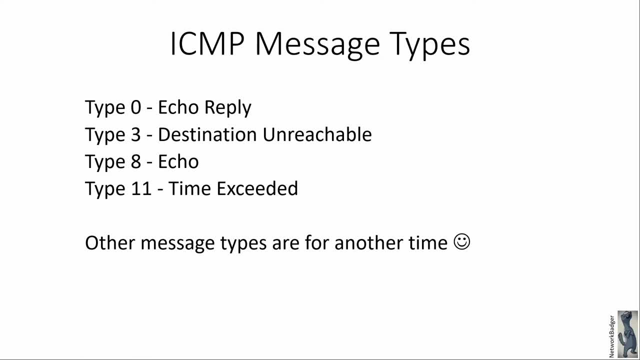 to your destination. you should be asking why that? that's a lot. so if your ping runs out of hops, that usually means one thing: routing loop. there is a router or a pair of routers misconfigured somewhere, or there's a broken dynamic routing protocol somewhere, causing your ping packet to go ping. 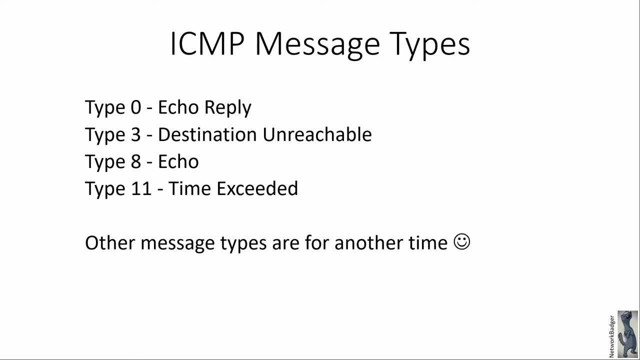 pong style between two routers right back and forth, or in a circle between three routers or more. that will guarantee you will quickly run out of your ttl hops and will never get to your destination right? so if you're receiving a time exceeded message, rest assured, there's a routing loop somewhere on the way between. 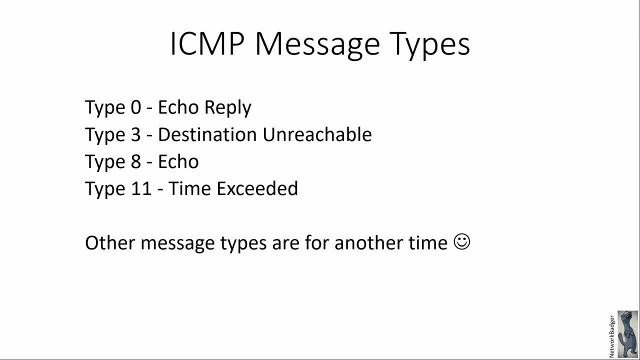 the source and the destination of your ping. so now we know how a ping is constructed in icmp echo request. so circuit Week or 00, away from diligentes. that's the number 1 way to process a timelapse. we've tries to save the workflow of which is really important. 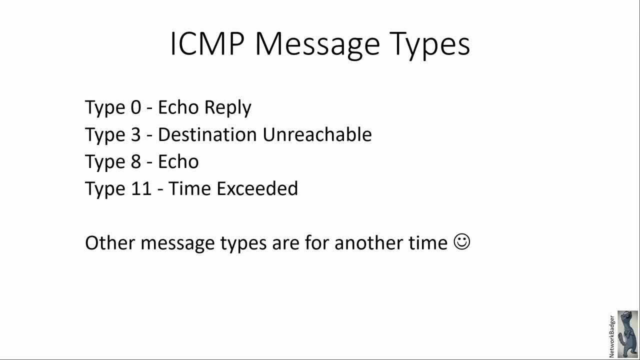 but we have to think about this a little bit more. just imagine if you encounter a speedgh- that one it's right around the center of the highway- is that you need to change your timelapse window, like the one that you are seeing right now? so if you have a primed been the utility that we've used for民ю. 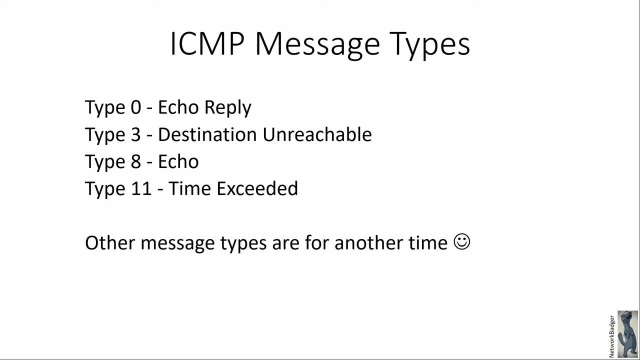 encounter to discard our packet. when discarding the router will return an icmp error message- time exceeded and we will want only one thing from that message: the ip address of the router that sent the error message. we will write down the ip address of the router that discarded our. 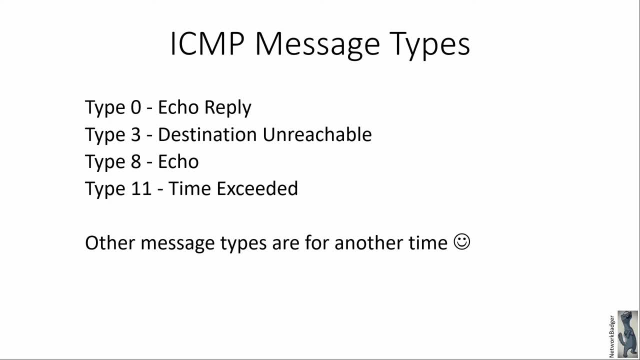 initial echo request and will repeat the process. now, setting our ttl value to 2, we expect the second router to drop our message as well and reveal its ip address, and so on. we will keep incrementing ttl by one until we reach the final destination. eventually, we will receive the echo. 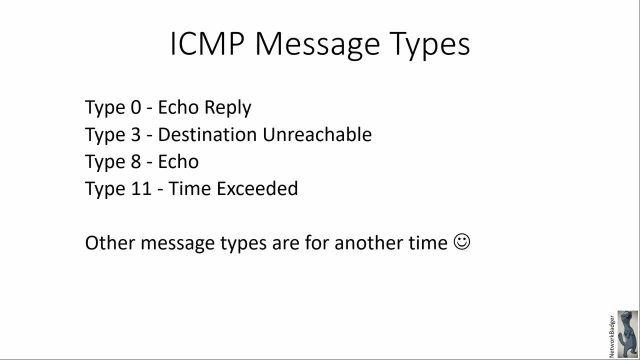 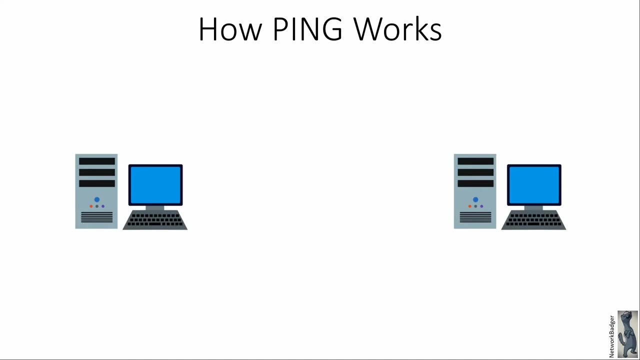 reply message and that will conclude our trace route right. so the trace route is just a series of pings with time to live value incrementing by one. so let's see on a quick animation how ping works. pretty straightforward. our pc on the left will generate an echo request. 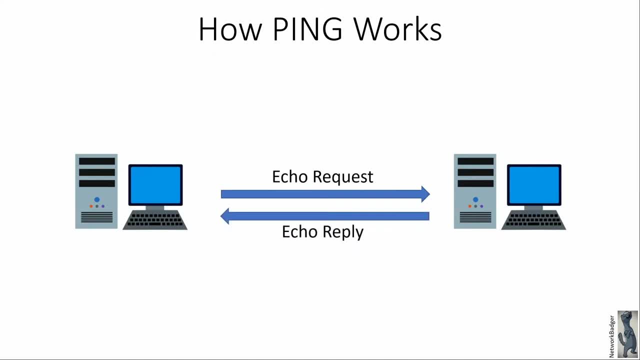 that will reach the pc on the right and, if everything goes well, the pc will generate a reply. we'll receive it. that concludes our ping. this is a very small network, probably a land local network, but it doesn't matter. these computers may be in the same room or they may be. 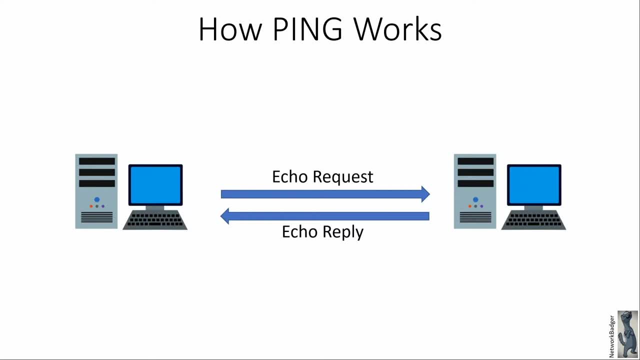 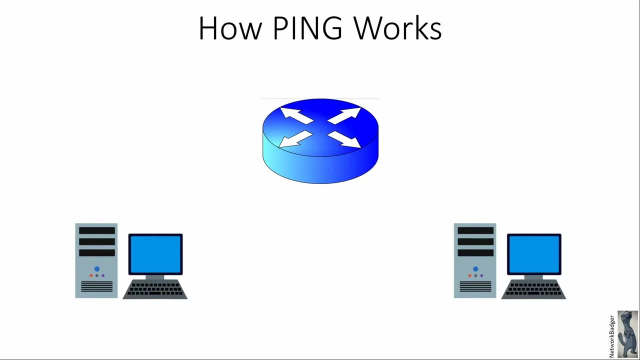 half the world apart. it doesn't matter, this process will work the same. there may be routers in between right, so let's insert a router. complicate our topology a little bit. so we're inserting router between our computers and let's imagine our ping is a little broken. 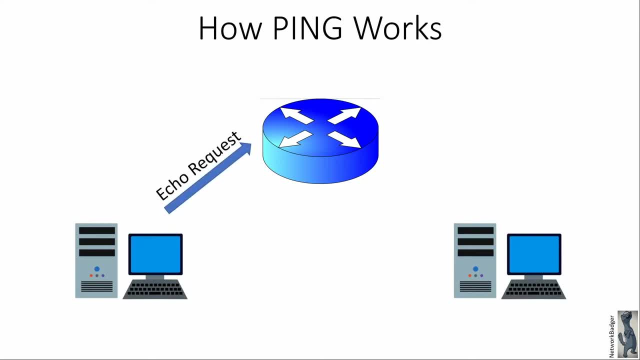 time. so again we start with an echo request. it goes from the computer to the router. this router is directly connected to the PC on the right, but there's something broken. so this router knows that in order to reach the PC on the right, it would have to send out the packet out of the interface on the right. 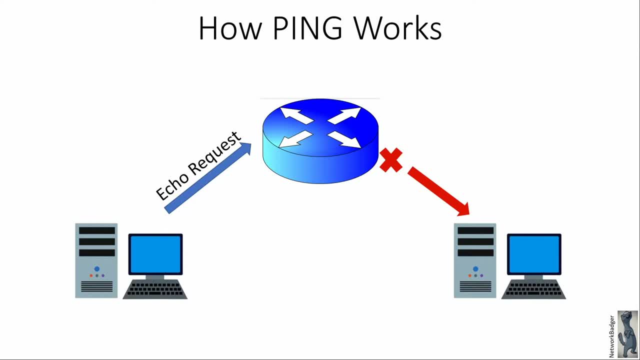 but that interface happens to be down. so the router knows that the only way to get to the computer is unusable. the router knows that for sure, because the computer is directly connected to the router. so the router will behave nicely. try to be helpful and the router will originate and generate an error message. 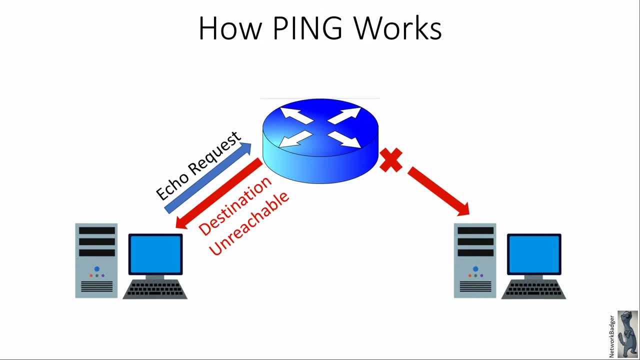 for us. destination unreachable message. ICMP error message. so we will learn from that message that well, oh well, we cannot ping the device. the device is unreachable. by the way, nobody asked this router for any input right. the computer on the left was asking a question, was asking something to the computer on the right- nobody. 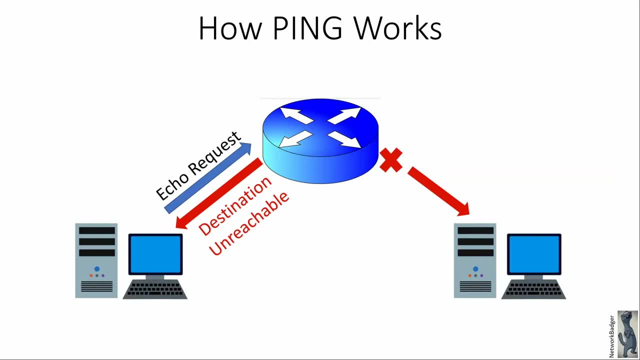 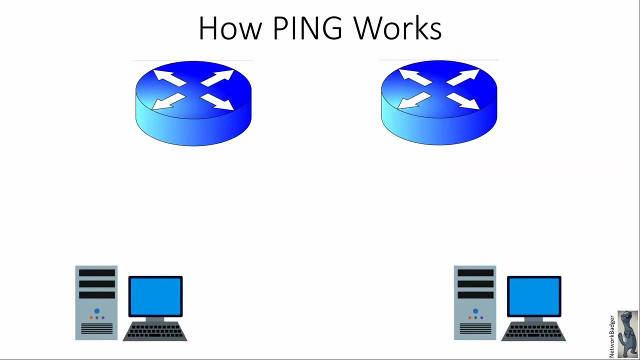 asked the router, anything but the router figured. it's a nice thing to do to get involved and tell us that we won't be able to reach the computer on the right. so that is our ICMP message destination unreachable. adding another router into our topology here, this time we will. 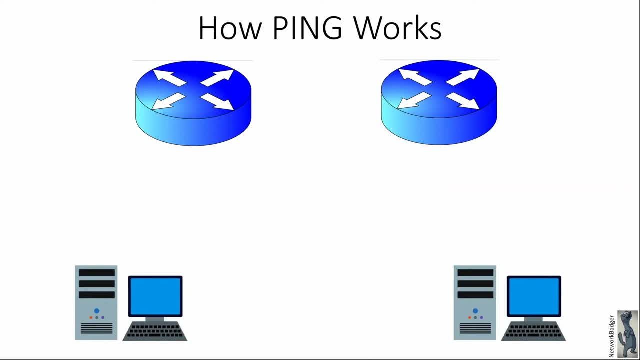 imagine that these two routers are misconfigured. actually, the router on the right is misconfigured, the second router is misconfigured, so we're sending our echo request. our ping reaches the first router successfully, which is the second router successfully. now the second router should be forwarding that ping. 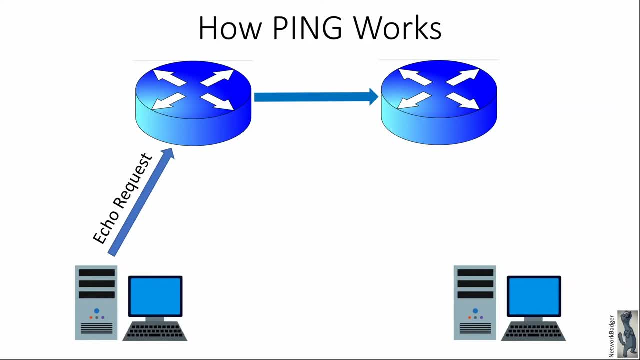 packet to the destination, to the computer on the right, but there's something that's configured to the router: instead of sending the packet to the destination, sends it back to the first一个. so this is our routing loop. here and the long burn is truer, and here because that parameter S copies it with miss ееpy. so let's cover it up and plug it in. 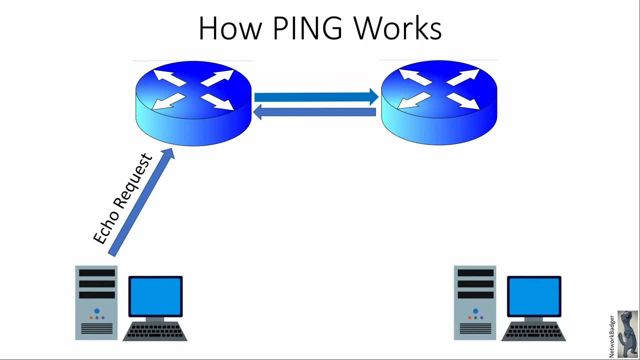 And this way we will run out of hops, Detail value will go to zero And we will receive the time exceeded error message. So our ping will never reach the destination And it's the fault of the router. So there's nothing wrong with our destination, but there's no path to it. 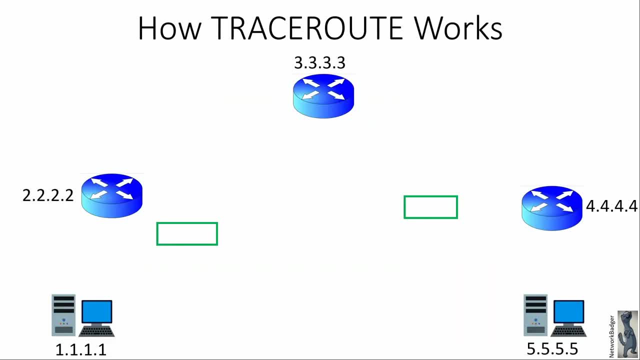 And now let's look at a quick and simple trace route. animation, Simple topology. We have two computers, Computer 1 and computer 5. Right, Bottom, left and bottom right. We will be sending a trace route from computer number 1 to computer number 5.. 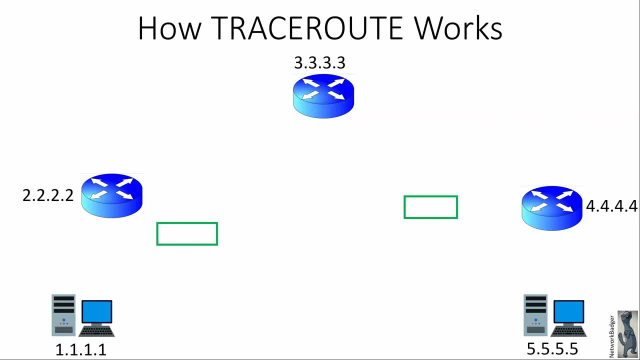 And our trace route will start. This is a regular echo request And our initial time to live is set to 1.. So we want to focus on this time to live value here And now. we will focus on the reply. The first router will respond saying time to live exceeded. 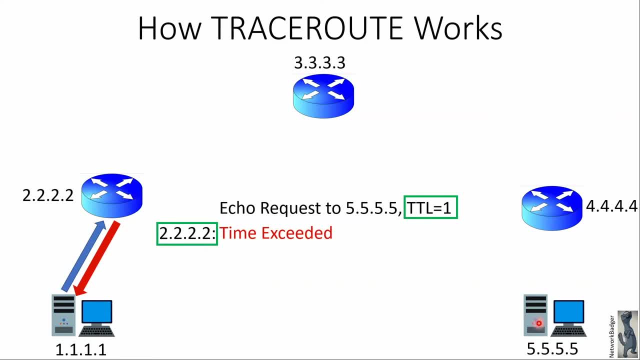 The first router knows how to reach the ultimate destination, But he's not allowed to proceed because the time to live was so low. the first router that received the packet had to discard it. So the first router responds back to us saying sorry, time exceeded. 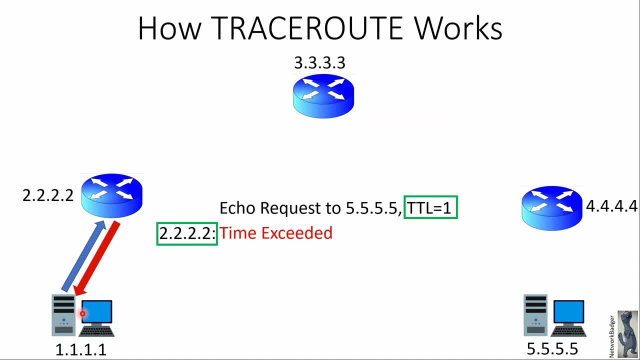 Just like on the previous slide, Time exceeded. But we expect that And we expect the time exceeded message from the first router. In fact, all we care about we want to see his IP address. That's all we need. We intentionally set our TTL to 1.. 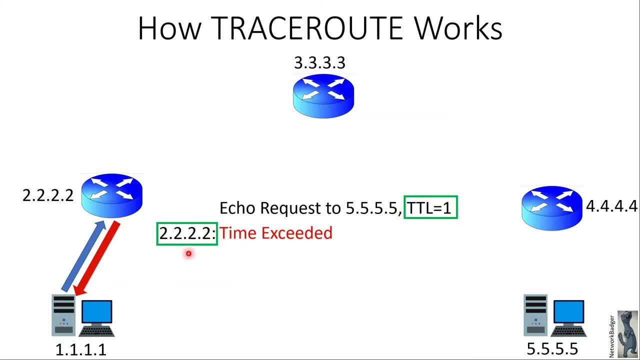 Because we want to capture the IP address of the device that will send us the expected error message. Moving on, Now we set our TTL to 2.. Our second attempt: We increase our TTL by 1.. Now it's 2.. And again we know we will receive an error message from the second router. 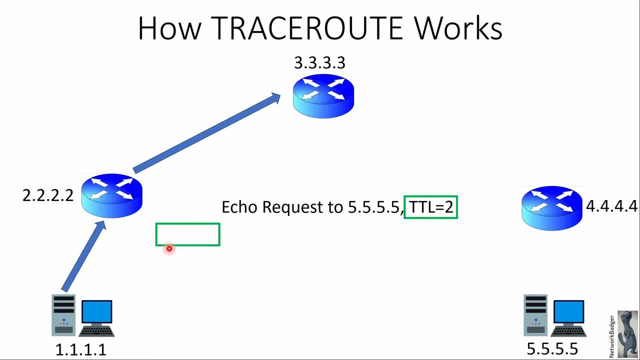 All we want is an error message. All we want is the IP address of the second router. And here it is. The error message comes back: Time exceeded. So this router doesn't know that we're doing a trace route. This router doesn't know, doesn't care whether we're doing a ping or a trace route or it's a regular IP packet. 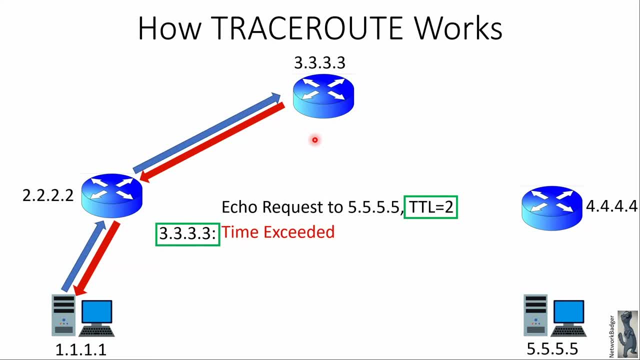 All this router knows is that it received an IP packet with time to live expired, So it responds. We capture his IP address, Repeat. Now we increment our TTL to 3. Same thing: We're getting the error message from the third router. 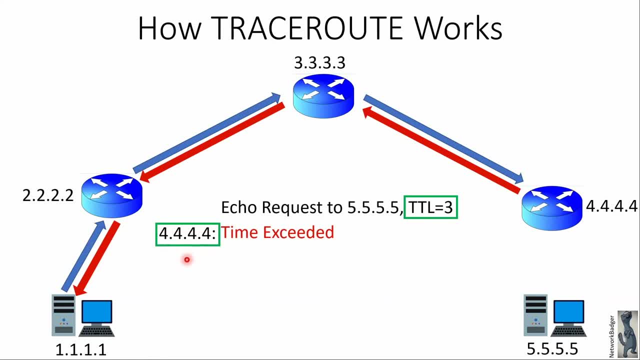 Router 4.4.4.4.. And next time we, when we set our TTL to 4, we actually reach, we reach our computer And our computer will respond with an echo reply And we know it comes from 5.5.5.5.. 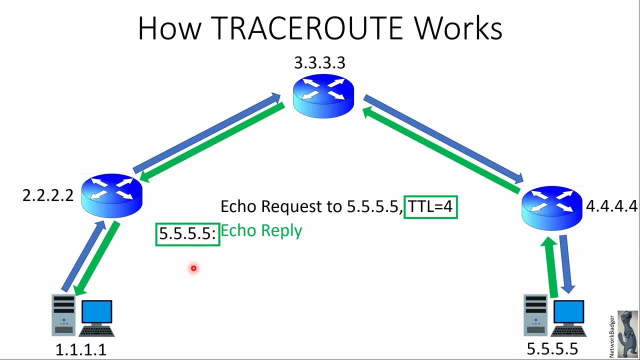 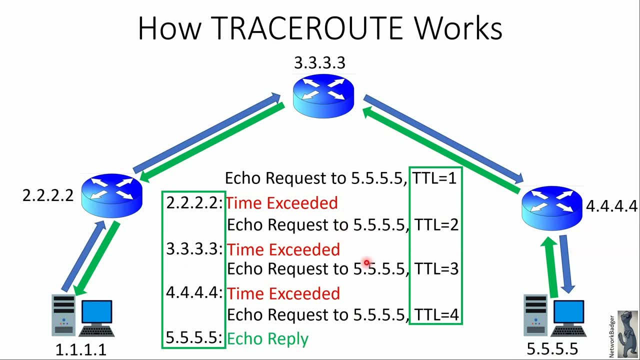 That's what we were initially trying to ping our trace route to. So the whole picture will look like this: In 1,, 2,, 3, and 4 steps, So 4 hops here. We increased our TTL from 1 to 2 to 3 to 4.. 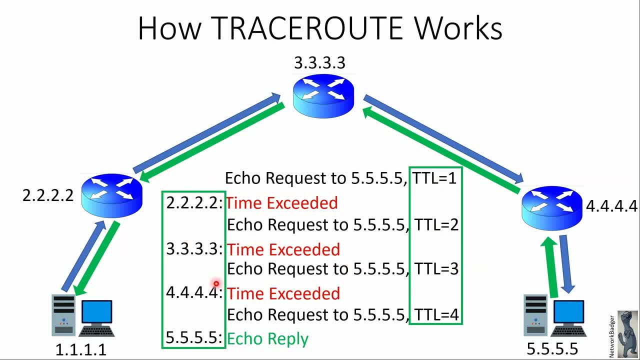 We have accumulated this little List of IP addresses on the left side. This list of IP addresses is our trace route. So we can say tracing from 1.1.1.1 to 5.5.5.5 took us 4 hops. 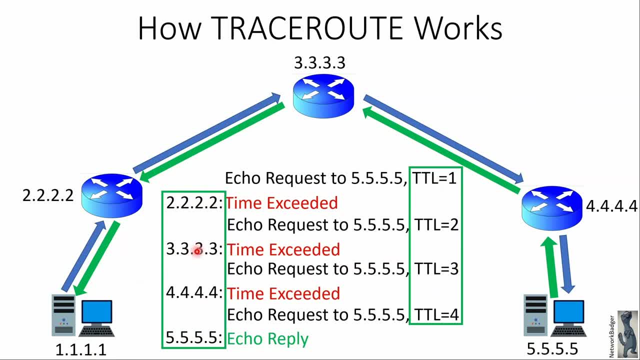 The first hop was 2.2.2.2.. The second hop was 3.3.3.3., 4.4.4. And 5.5.5.. This is our trace route. So we built our trace by manipulating two message types. 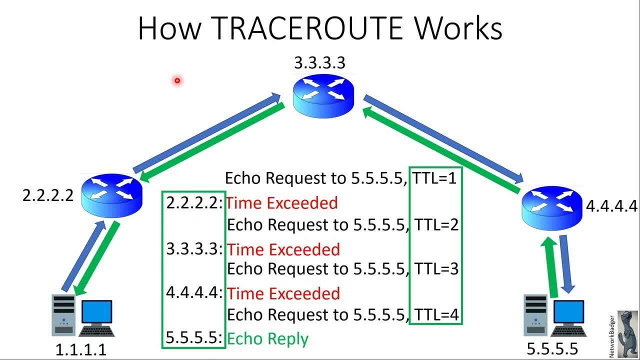 Echo request and time exceeded. So that's how ping and trace route work in principle. And now let's look at some real pings and trace routes. 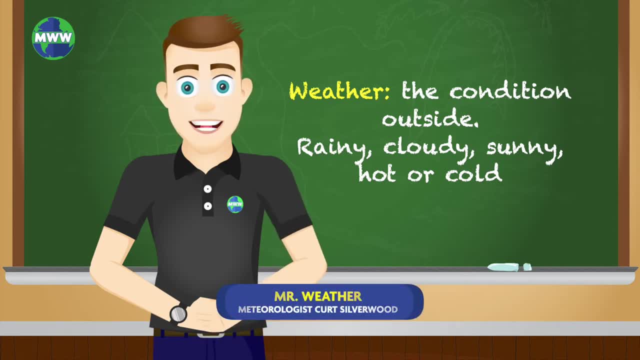 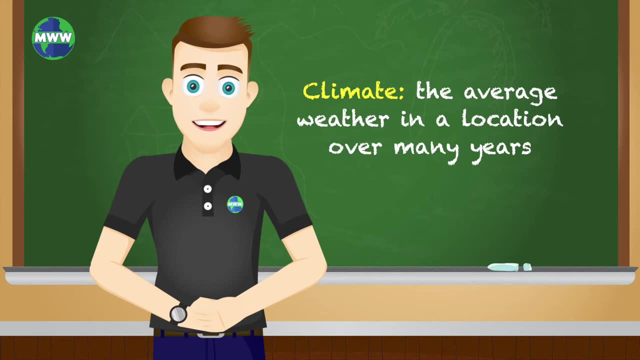 Each day we experience weather. The condition outside, whether it's rainy, cloudy, sunny, hot or cold Climate, is the average weather in a location over many years. It can take hundreds, thousands or even millions of years to see any type of change in climate. 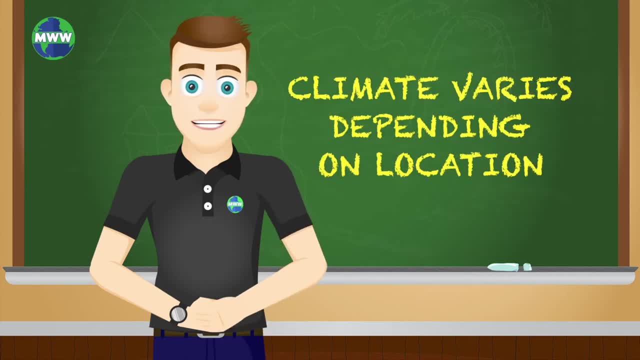 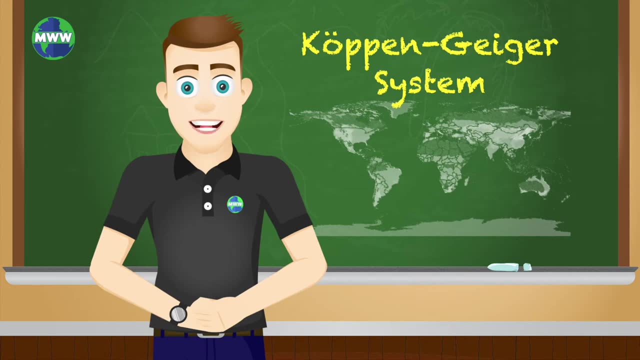 Depending on location, climate varies and is categorized into different climate zones. The Köppen-Geiger system, developed at the end of the 19th century, is the most commonly used system to determine climate zones. There are six zones: Zone A- tropical moist climates. Zone B: 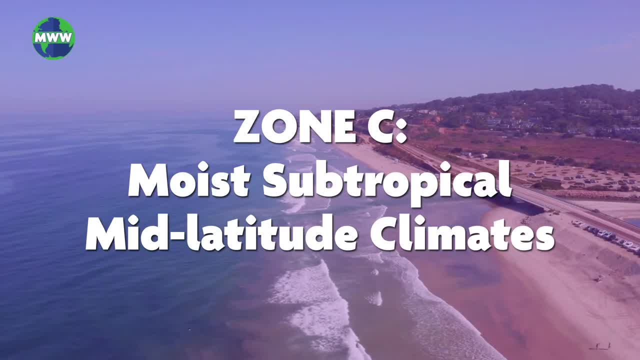 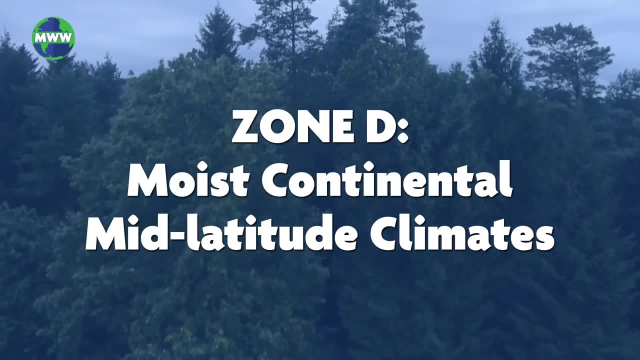 dry, arid climates. Zone C- generally warm and humid, a moist subtropical mid-latitude climate. Zone D- moist continental mid-latitude climates with warm to cool summers and cold winters. Zone D- moist continental mid-latitude climates with warm to cool summers. 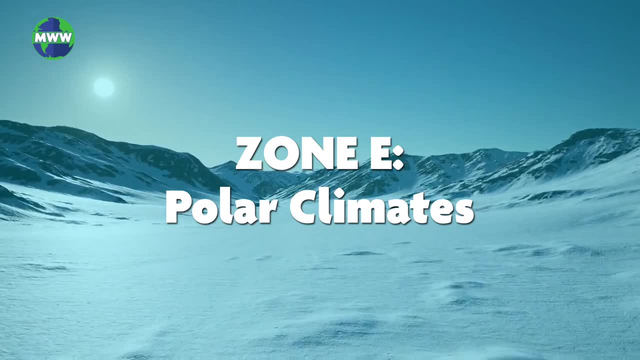 and cold winters. Zone C: generally warm and humid, a moist subtropical mid-latitude climate. Zone D: moist continental mid-latitude climates with warm to cool summers and cold winters. Zone E: polar climates with cold temperatures year round. Zone H: highland climates that are unique based on elevation. 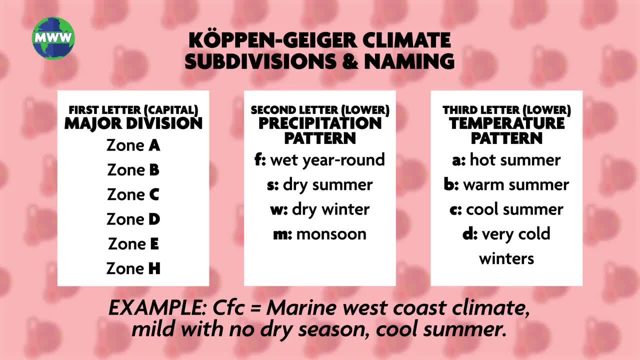 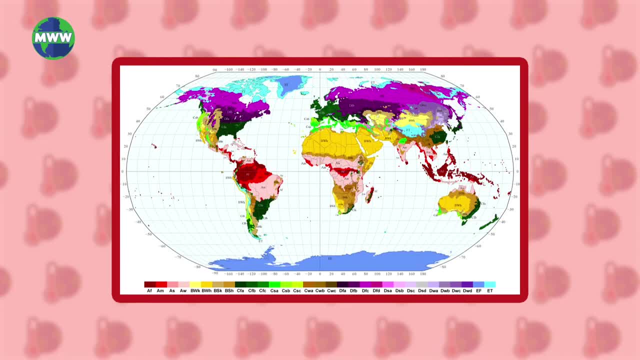 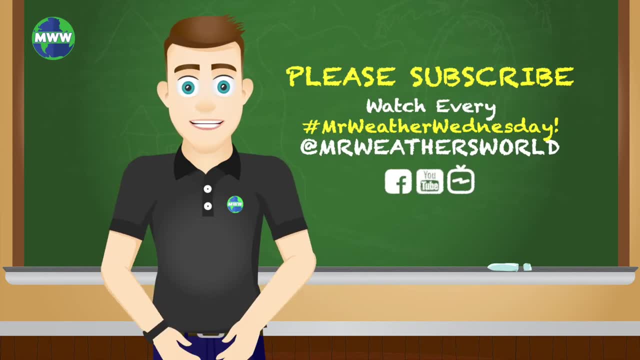 causing rapid changes over short distances. Each of these zones are further divided into smaller groups based on precipitation and temperature patterns. On a map, each zone is represented by different colors. Next time, catch the monthly What's What. Thank you for watching and please subscribe to Mr Weather's World on YouTube for new videos.